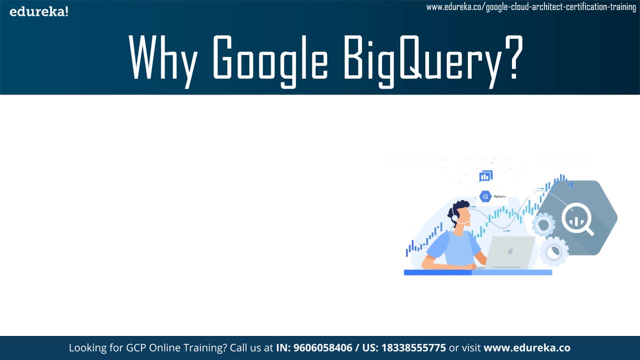 Now BigQuery is a GCP serverless, highly scalable and cost-effective cloud data warehouse. It provides both batch and streaming modes to load data. It also allows importing data directly as a service application using BigQuery data transfer service. Second is ease of implementation. 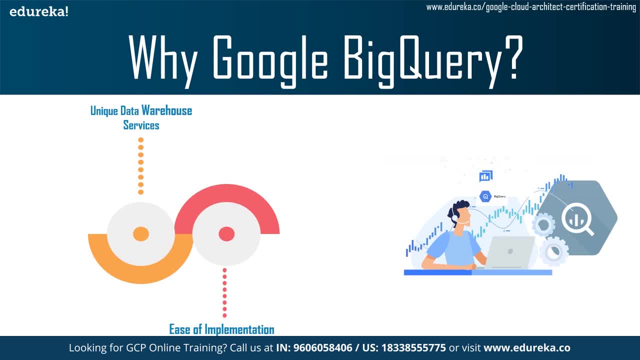 So building your own is expensive, time-consuming and difficult to scale. Now with BigQuery, you need to load data first and pay only for what you've used. Third is its speed. Now it processes billions of rows in seconds and handle real-time analysis of streaming data. 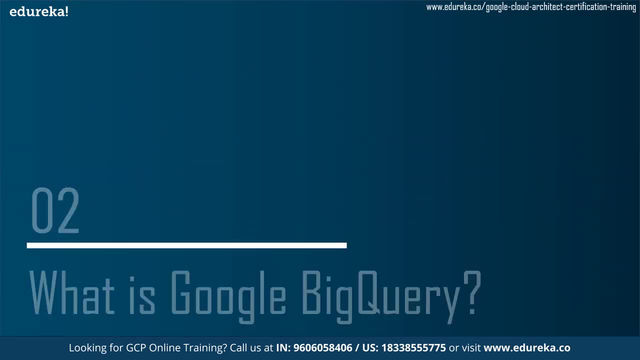 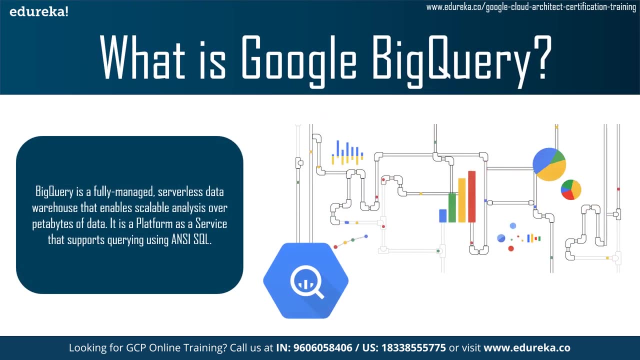 Now that you have understood why we need BigQuery, let us now understand what actually is BigQuery. So BigQuery is a fully-managed, serverless data warehouse that enables scalable analysis over petabytes of data. It is a Platform as a Service that supports querying using ANSI SQL. It also has built-in 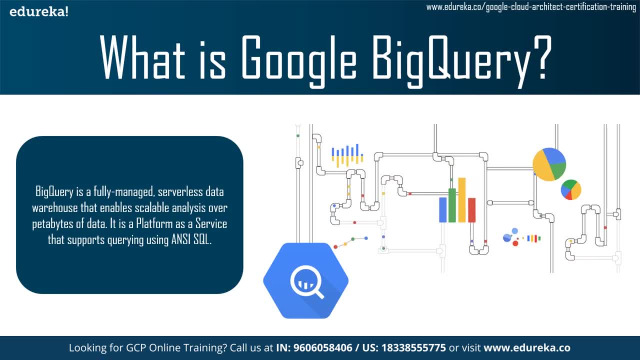 machine learning capabilities So you can build an operationalized machine learning solution using simple SQL. You can easily and securely share insights within your organisation And beyond as dataset queries, spreadsheets and reports. BigQuery allows organisation to巩re because it's simple and easy to use. When a click-through is a release to all the. Career Control. Our Dataу and data гол prefab mandats are also quite straightforward. The whole page of thecendashbye aspotty, necessary and clean description. bpn portion streaming file which I think the clients feel that's a bit. uniries are few each other. 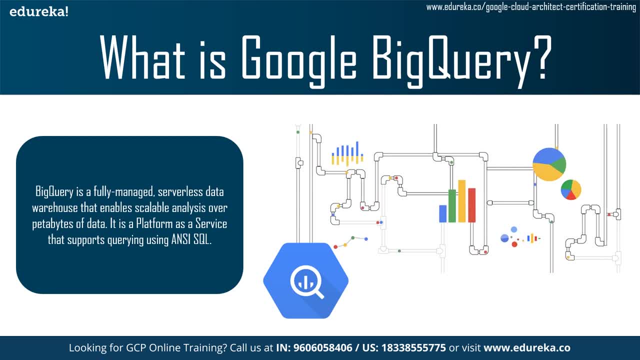 to capture and analyze data in a real time using its powerful streaming injection capabilities, so that your insights are always current, and it's free for up to 1 terabytes of data analyzed each month and 10 gigabytes of data stored. BigQuery serves managers underlying software as well as. 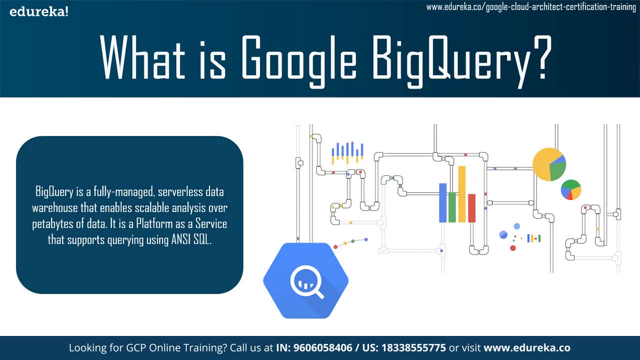 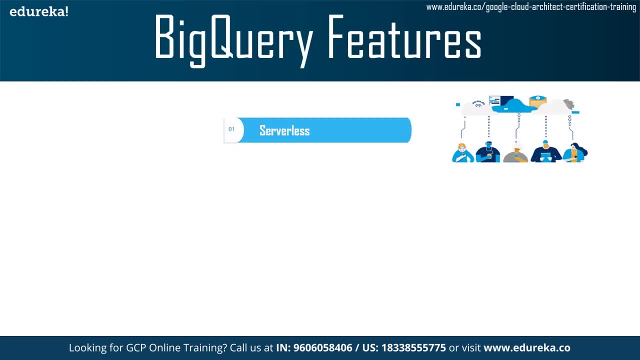 infrastructure, including scalability and high availability. Now let us look at some of the key features of BigQuery Now. first of all, it's serverless, So serverless data warehousing gives you the resources you need when you need them. with BigQuery, You can focus on your data and analysis rather than operating. 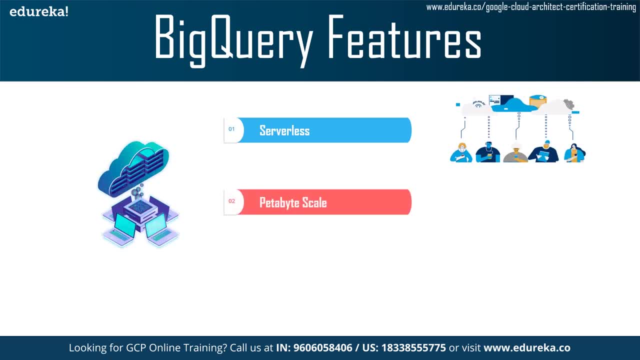 and sizing computing resources. So second is petabyte scale. BigQuery is fast and easy to use on data of any size. with BigQuery you will get great performance on a data while knowing you can scale seamlessly to store and analyze petabytes more without having to buy more capacity. Now third is a real-time. 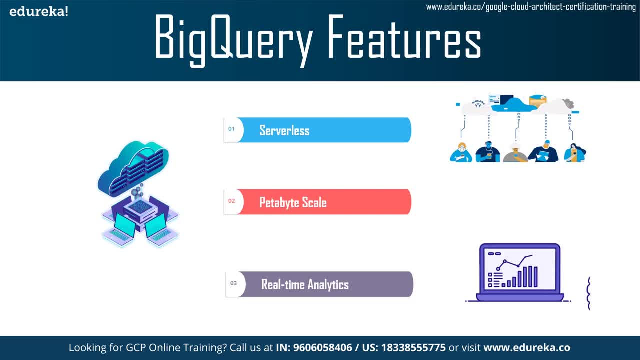 analysis, So you can have a better understanding of your data, and also analytics, So BigQuery's high-speed streaming injection API provides a powerful foundation for real-time analytics. Now BigQuery allows you to analyze what's happening now by making your latest business data immediately. 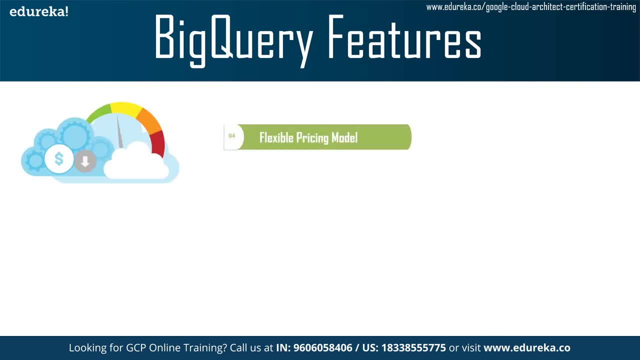 available for analysis. Fourth is flexible pricing models. So BigQuery enables you to choose the pricing model that best suits you. Now, on-demand pricing lets you pay only for the storage and computation that you use. Now we have the flat rate pricing, which enables 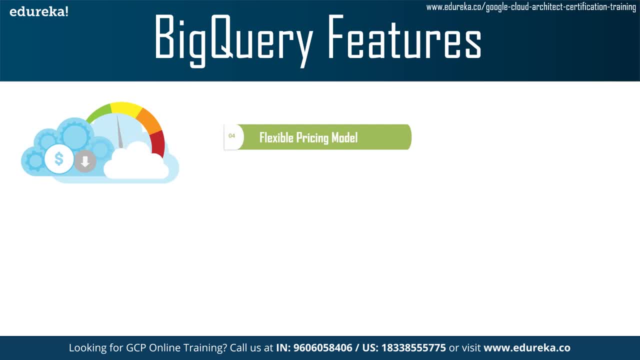 high-volume users or enterprise to choose a stable monthly cost for analysis. Now fifth is automatic. high availability- Now free data and compute replication in multiple location means that your data is available for query even in the case of extreme failure modes. Now BigQuery, transparently and automatically. 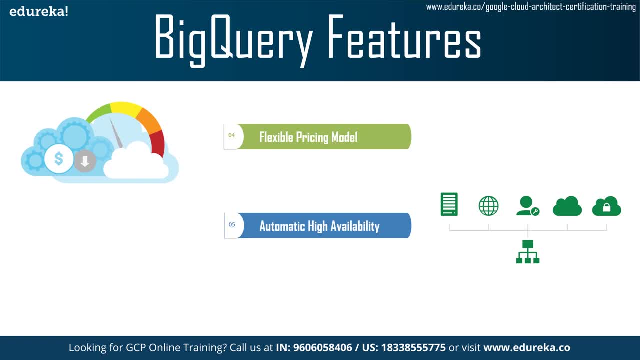 provides durable replicated storage and high availability with no extra charge and no additional setup. Sixth one is your data encryption and security. Now you have full control over who has access to the data stored in BigQuery. Now BigQuery makes it easy to maintain strong security with fine-grained. 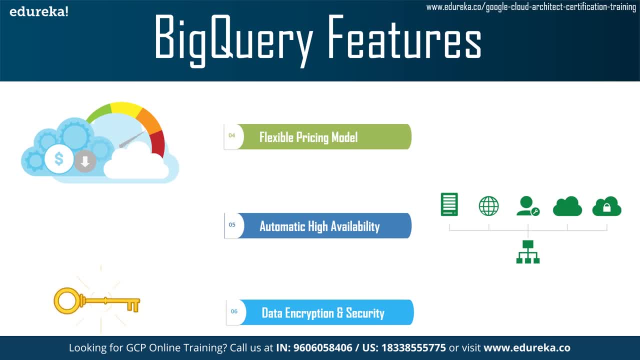 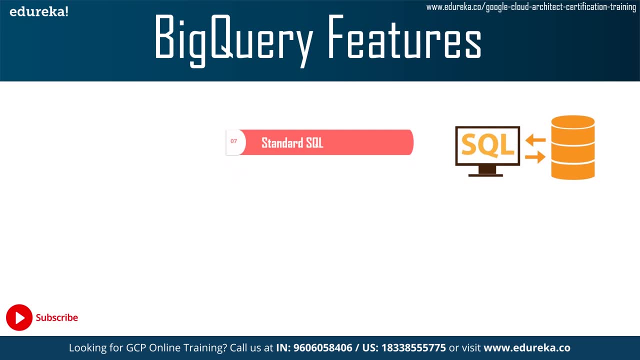 identity and access management, And your data is always encrypted, address and in transit. Seventh is BigQuery support a standard SQL dialects that is ANSI 2011 compliant, reducing the need for code rewrites and allowing you to take advantage of advanced SQL features. Now BigQuery also provide free ODBC and JDBC drivers. 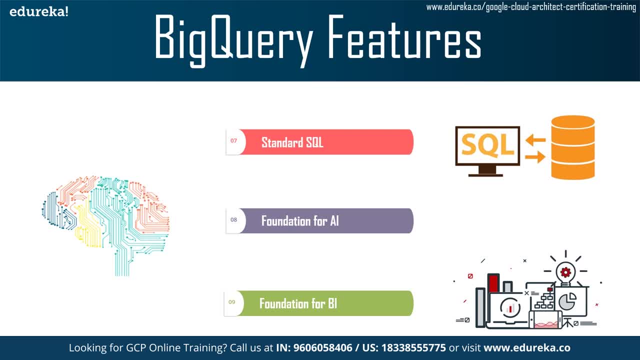 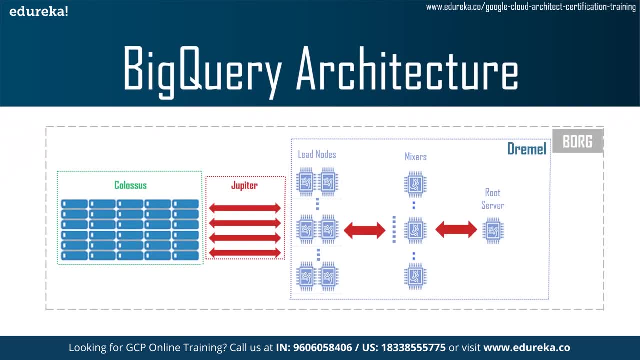 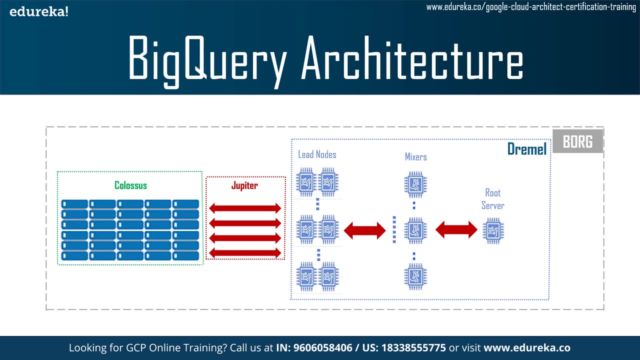 To ensure your current application can interact with BigQuery powerful engine. Let's now deep dive into BigQuery and have an architectural understanding of it Under the hood. BigQuery employs a vast set of multi-tenant services driven by low level Google infrastructure technologies like Dremel, Colossus, Jupyter and Borg. 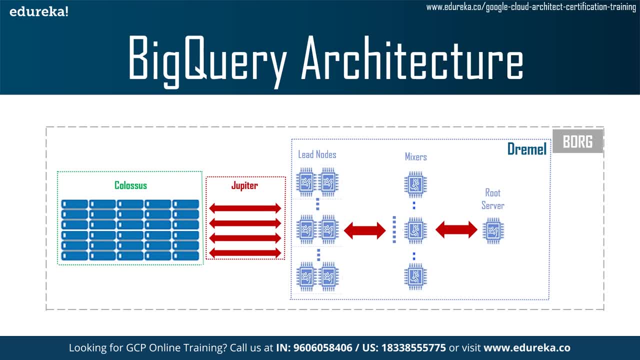 It takes more than just a lot of hardware to make your query run fast. BigQuery requests are powered by the Dremel query engines, which or just rate your query by breaking it up into pieces and reassembling the results. Now Dremel turns your SQL query into an execution tree. Now the leaf of the trees. 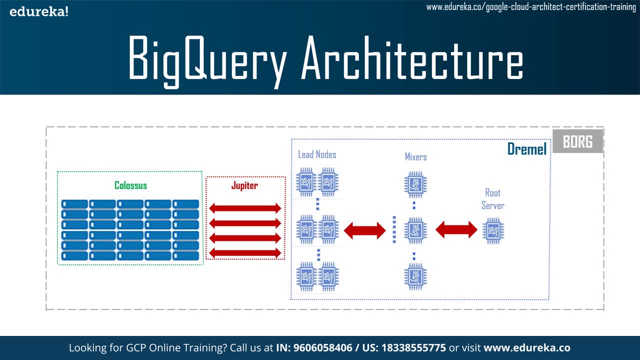 it's called slots, and do the heavy lifting of reading the data from Colossus and doing any computation necessary. The branches of the trees are mixes which perform the aggregation in between This shuffle, which takes advantage of Google's Jupyter network to move data extremely rapidly from one places to another. 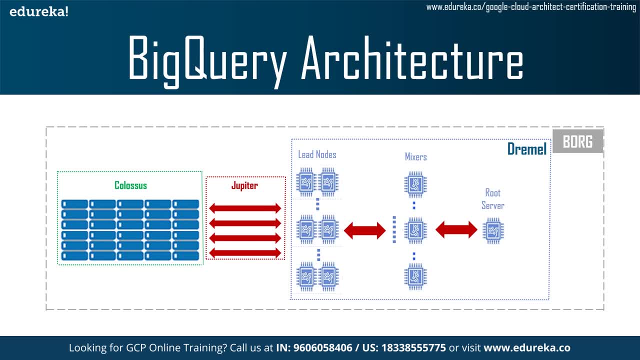 The mixes and slots are all run by Borg, which doles out hardware resources. Dremel dynamically appoints slots to query on and, as needed, Bases maintaining fairness among multiple users who are all querying at once. Now, a single user can get thousands of slots to run these queries. Dremel is widely used at Google. 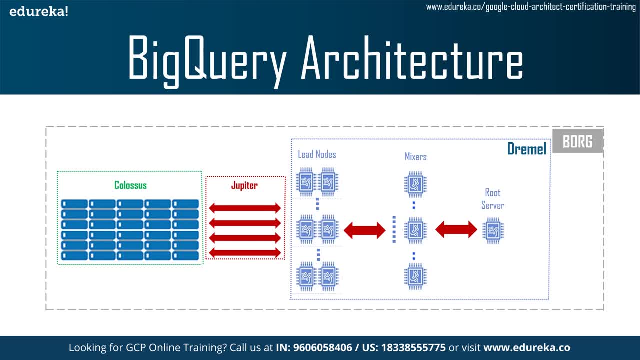 from search to ads, from YouTube to Gmail. So there is a great emphasis on continuously making Dremel better. Big query users get the benefit of a continuous improvement in performance, durability, efficiency and scalability, without downtime and upgrades associated with traditional technologies. Also big 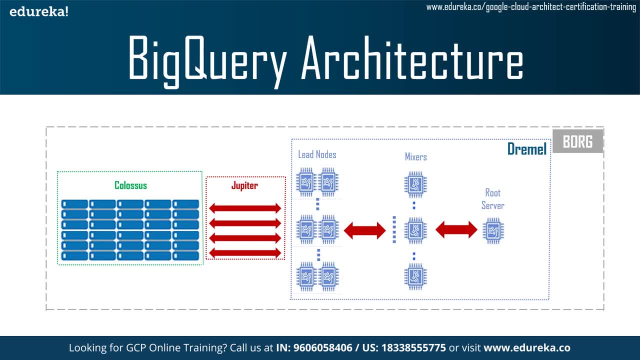 query relies on Colossus, which is Google latest generation distributed file system. Now each Google data center has its own Colossus cluster and each Colossus cluster has enough disks to get every big query user, thousands of dedicated disks at a time. Colossus also handle replication. 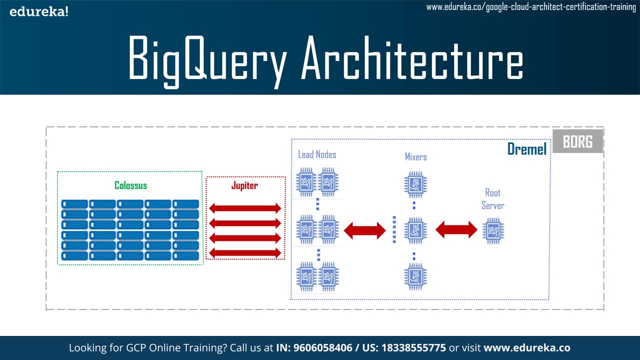 requirements. Colossus is fast enough to allow BigQuery to provide similar performance to many in-memory databases, but leveraging much cheaper yet highly paralyzed, scalable, durable and performant infrastructure. BigQuery leverages the column input output storage format and compression algorithm to store data in Colossus in the most optimal way for leading large amount of. 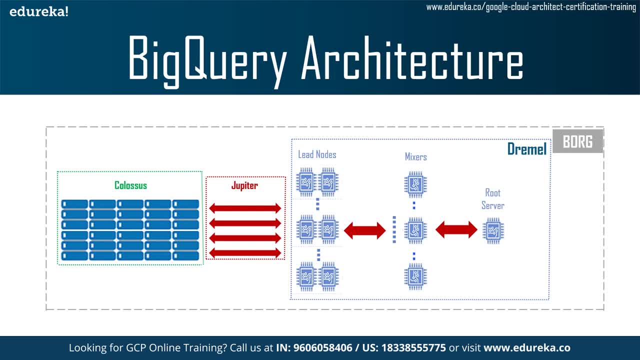 structured data Colossus allow BigQuery user to scale to dozens of petabytes and storage seamlessly without paying the penalty of attaching much more expensive compute resources, Typically with most traditional databases, to give you thousands of CPU codes dedicated to processing your tasks. BigQuery takes 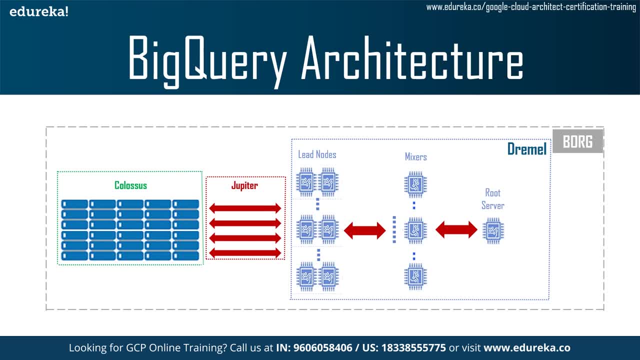 advantage of Borg, which is Google's large-scale cluster management system, For Colossus runs on dozens of thousands of machines and hundreds of thousands of cores. So your query, which use three thousand three hundred CPUs, only use a fraction of the capacity reserve for BigQuery and BigQuery. 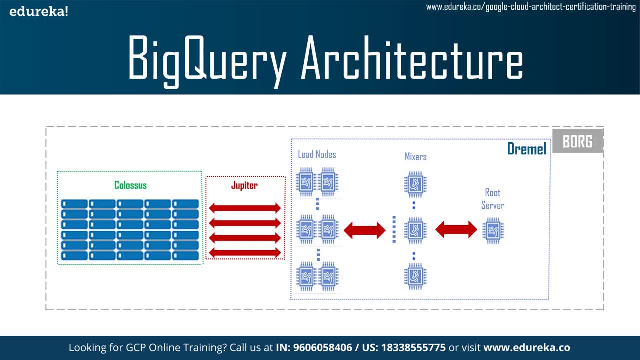 capacity is only a fraction of the Borg cluster. Borg assigns server resources to jobs. Now the job in this case is the driven cluster. machines crash, power supplies fails, network switch dies and any rate of other problems can occur while running a large production data center, Borg's roots around it and the 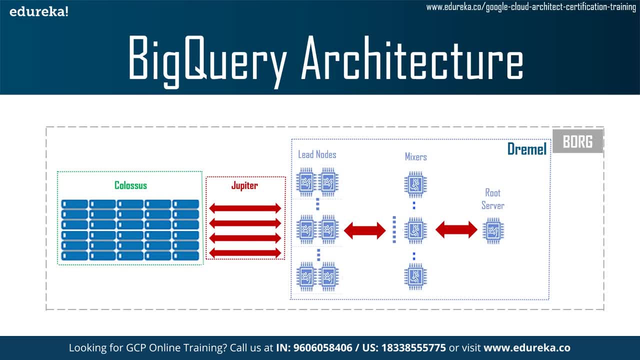 server layer is abstracted At Google scale, thousands of server will fail every single day and Borg protect us from the failures. Say, someone unplugs a rack in the data center in this middle of running your query and you will never notice the difference. beside obvious needs for resource coordination and compute resources, Big data workloads, 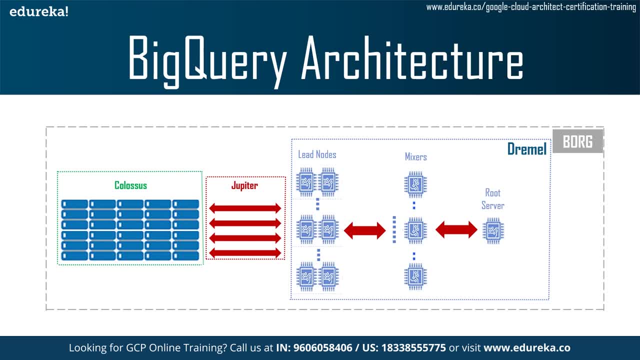 are often throttled by networking throughputs. Google Jupyter network can deliver one better bit per second of total by section bandwidth, allowing us to efficiently and quickly distribute large workloads. Now Jupyter networking infrastructure might be in the single biggest differentiator in Google Cloud. 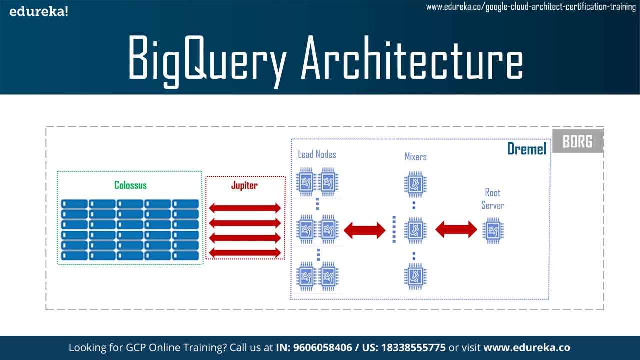 platform. Now it provides enough bandwidth to allow one lakh machines to communicate with any other machine at 10 gigabyte, The network bandwidth needed to run our query, which uses less than 0.1 percent of the total capacity of the system. Now this full duplex bandwidth means that locality within the cluster 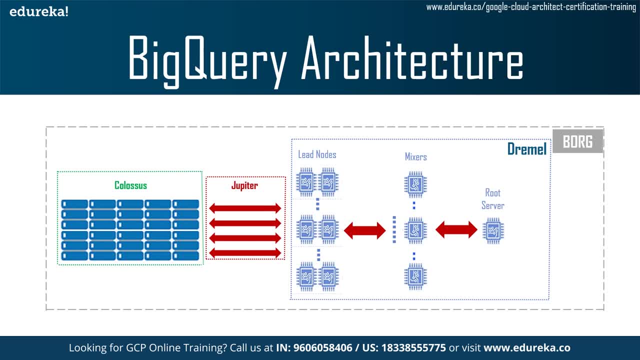 is not important. if every machine can talk to every other machine at 10 gigabytes per second, Racks don't matter. traditional approaches to separation of storage and compute include keeping data in an object store like Google Cloud storage or AWS S3, and loading the data on demand to virtual machines. Now. 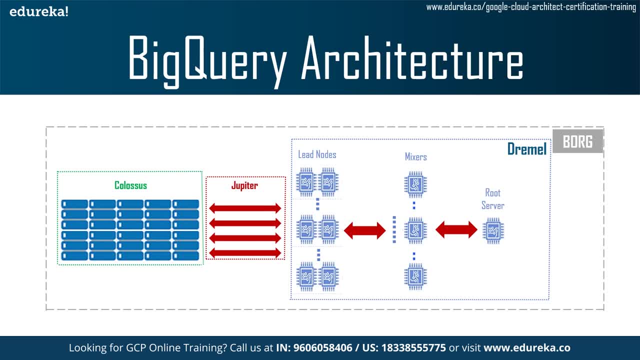 this approach is often more efficient than core tenant architectures like HDFS, but it's subject to local virtual machine and object storage throughput limits. Jupyter allows us to bypass this process entirely and read terabytes of data in second directly from storage for every SQL query. 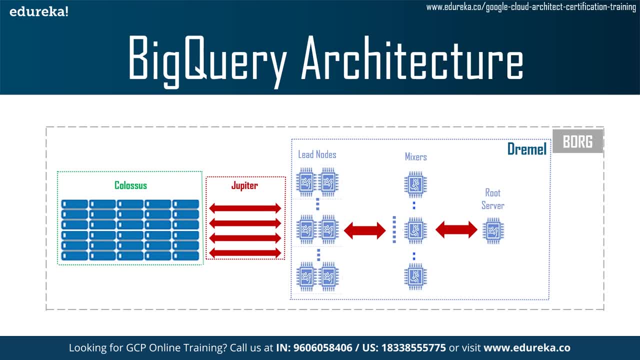 Now, in the end, these low-level infrastructure components are combined with several dozen high-level technologies, API and services like Bigtable, Spanner and Stubby to make one transparent, powerful analytics database: BigQuery. the ultimate value of BigQuery is not in the fact that it gives you 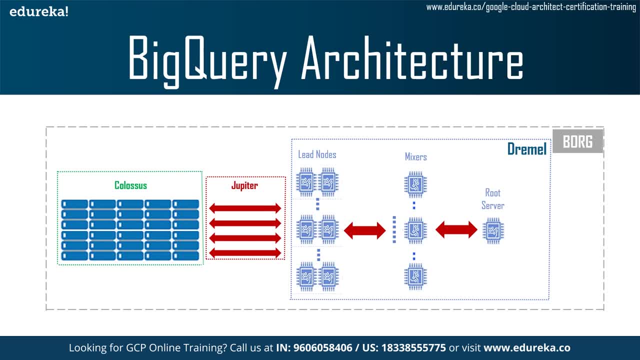 incredible computing skill. it's that you're able to leverage this skill for your everyday SQL queries without ever so much as thinking about the software, virtual machines, networks and tests. Now BigQuery is truly a serverless database, and BigQuery simplicity allows customers with 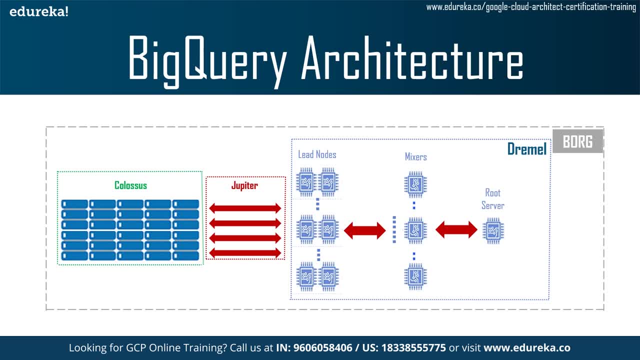 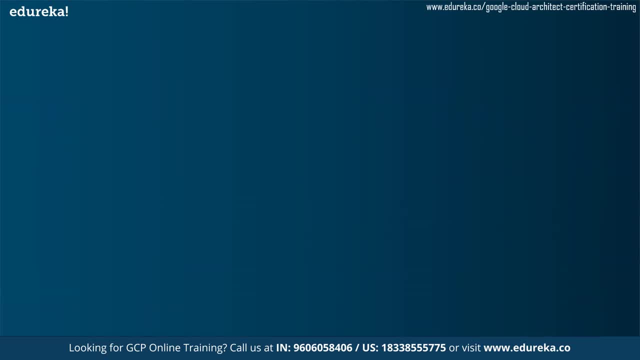 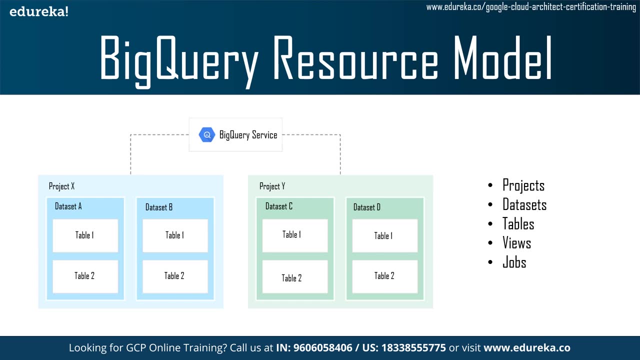 dozens of petabytes to have nearly identical experience, as it's free for our customers. Now that we have reviewed the high-level architecture of BigQuery, we now need to look at the BigQuery storage organization and format. Let's understand BigQuery resource model. 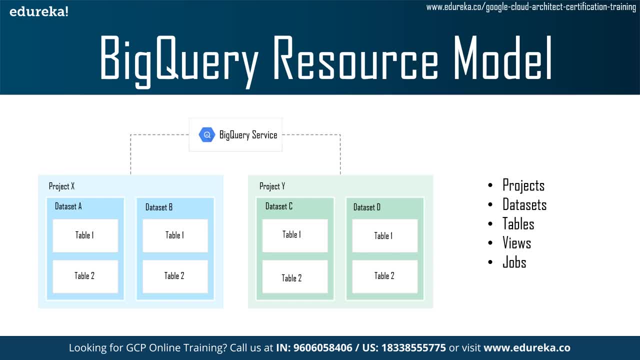 Now BigQuery organized data tables into units called datasets. Now these datasets are scoped to your GCP. Now these multiple scopes, project data sets and tables help you structure your information logically. Now you can use multiple data cells to separate tables pertaining to different analytic domains and you can use project level scoping to isolate. 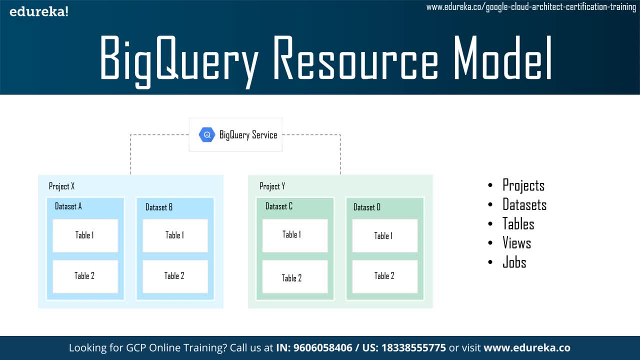 data sets from each other according to your business needs. So in this, the first one are projects. So projects are root namespace for objects which contain multiple data sets, job access, control lists and IEM roles. Now it's also control, billing users and user privileges. Now second is dataset, which is a collection. 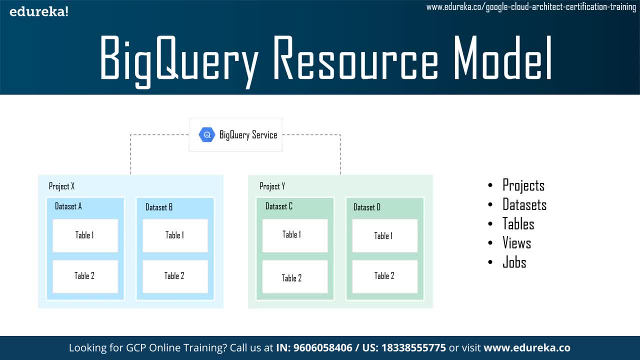 of related tables or views, together with labels and description. It allows access, control and dataset levels and define location of data that is multi-regional or regional. That is, if it is a multi-regional, it can have, like US or European Union or any other multi-region. 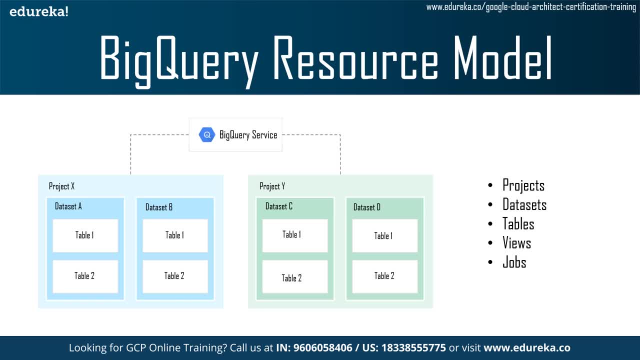 And if it is just regional, so it can be Asia Northeast, It specifically goes into the region. that's all Now. then there are tables, which are collections of columns and rows stored in managed storage and defined by a schema with strongly typed columns of values and also allow access control at table label and column label. 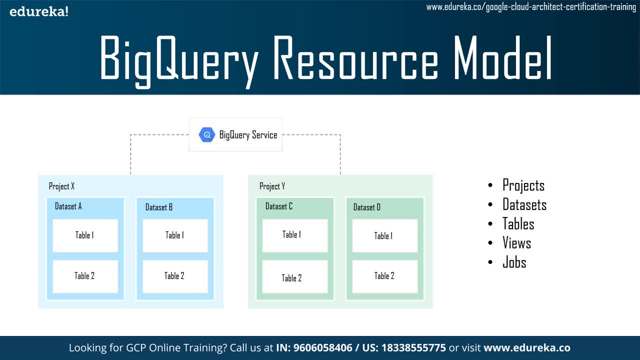 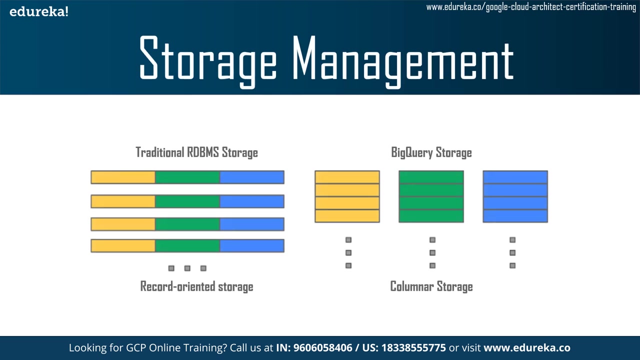 The next is views, so which are virtual tables defined by SQL query, and it allows access control at view level. And the last one is jobs. These are actions run by BigQuery. The next in this we have is a storage management. Now let's review how BigQuery manages the 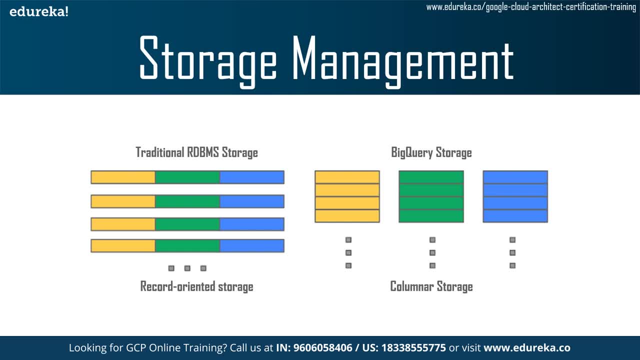 storage that holds your data. Traditional relational databases like MySQL stores data row by row, which means record-oriented storage. This makes them good at transactional updates, And OLTP means online transaction processing use cases. Now let's take a look at the storage management. The storage management is basically the same. 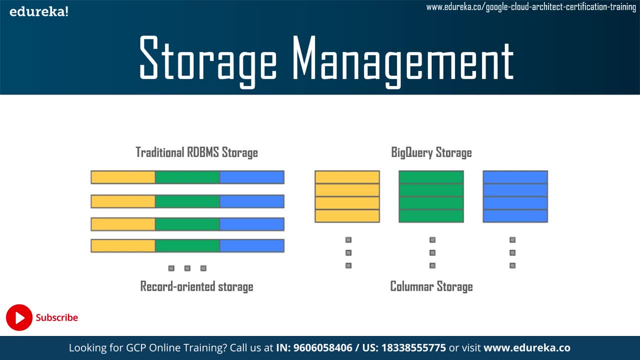 as the data storage management. The storage management is basically the same as the data storage management Then we have is BigQuery storage, Now BigQuery. on the other hand, use columnar storage, where each column is stored in a separate file. block This make BigQuery. 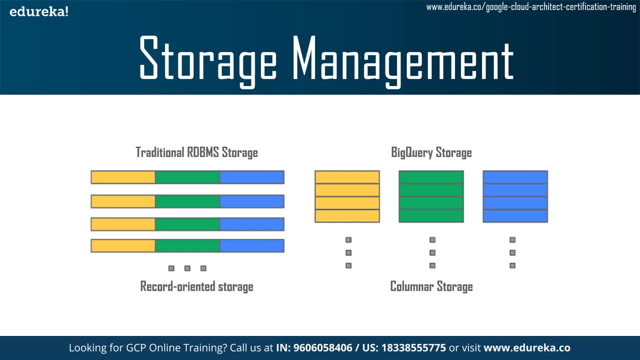 an ideal solution for OLAP, which means online analytical processing use cases. Now you can stream data easily to BigQuery tables and update or delete existing values. BigQuery support mutation without limits. Now mutation like insert, update, merge or delete BigQuery. 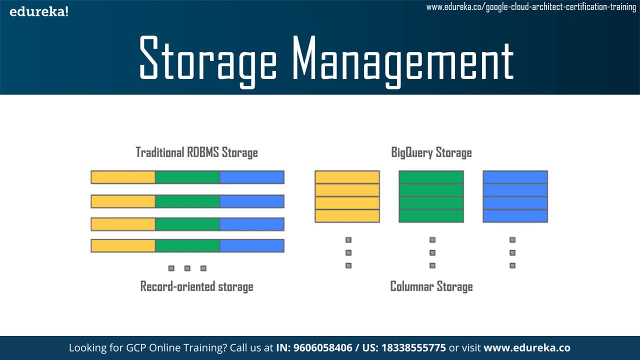 uses variation and advanced data storage. Now you can see that the data storage is a little bit slowowski starts matrix. that's why we want to include it in the 관�. It's ŞimdiAL aan Toyota 4K. 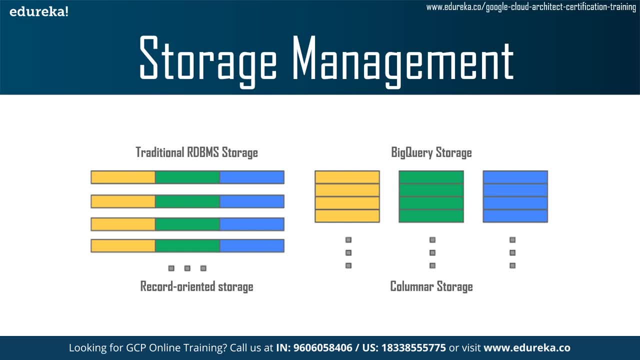 Until then. thank for taking a look. Alright, this before that. full introduction of BigQuery. here is full introduction to Alto BigQ In demo. we've gone throught the individual Watsonization functions. Here a table overview of Android OS gate. 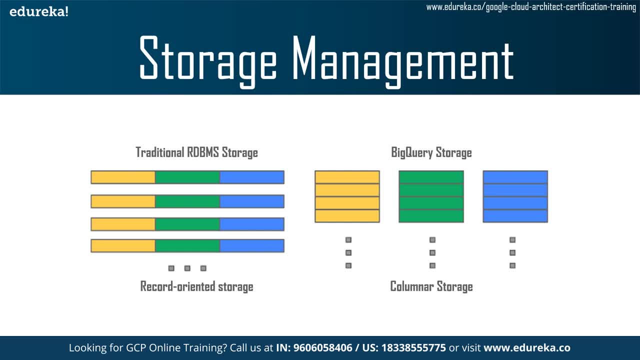 Android OS Circuit and instead we'll notice lots of frontend security. Fortunately, we've also babyn requirements. Thank you for your attention. capacitor file which are compressed and encrypted on disks. BigQuery uses query access patterns to determine the optimal number of physical charts and 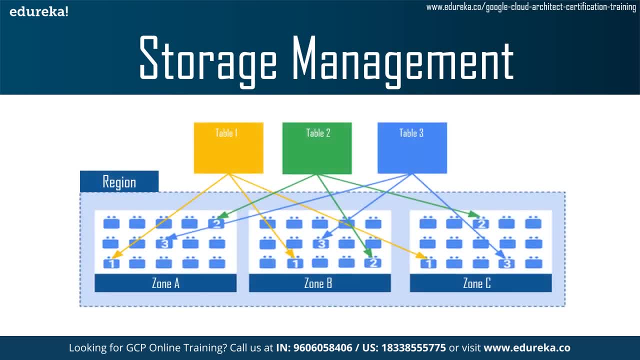 how data is encoded. The actual persistent layer is provided by Google Distributed File System, Colossus, where data is automatically compressed, encrypted, replicated and distributed. Colossus ensures durability, using Ensure encoding to store redundant chunks of data on multiple physical disks. 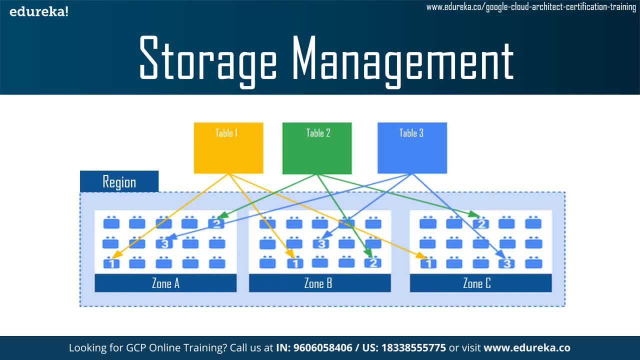 This is all accomplished without impacting the computing power available for your query. Separating storage from compute allows you to scale to petabytes in storage seamlessly without requiring additional expensive compute resources. There are a number of other benefits of decoupling compute and storage. 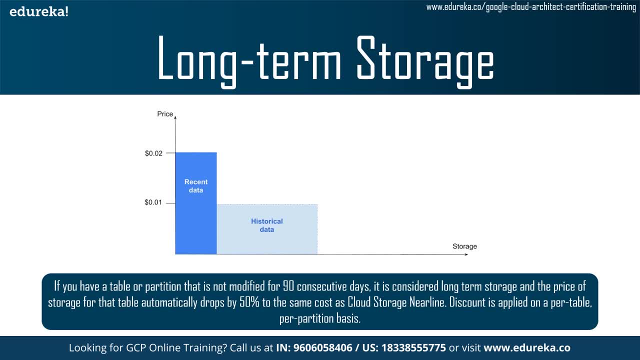 You can also take advantage of long-term storage. You can load data into BigQuery at no cost, because BigQuery storage costs are basically based on the amount of data. like the first NGP is free each month and whether the storage is considered active or long-term. 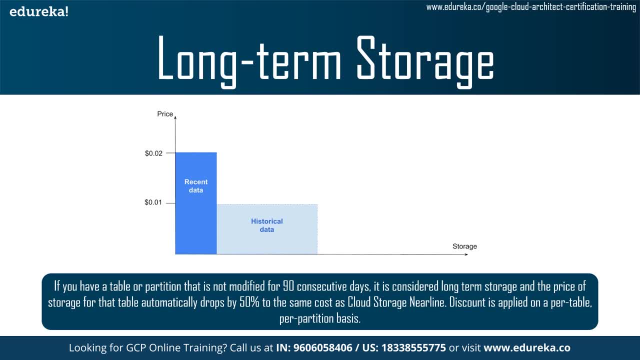 If you have a table or partition modified in the last 90 days, it is considered as active storage and incur a monthly charge for data storage at BigQuery storage rates. If you have a table or partition that is not modified for 90 consecutive days, it is considered. 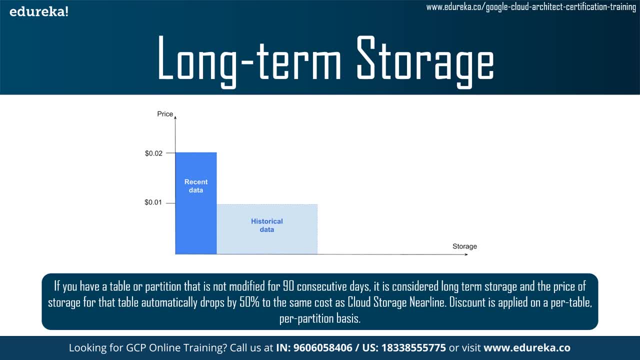 long-term storage And the price of storage for that table automatically decreases, So you don't have to worry about that. It automatically drops by 50% to the same cost as cloud storage near line. The discount is applied on a per-table, per-partition basis. if you modify the data in the table, 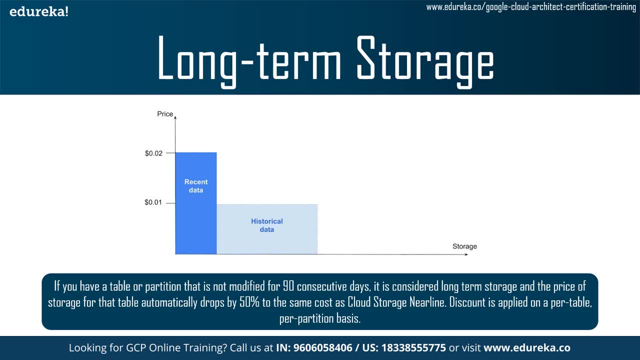 The 90 days counter then resets. Best practice when optimizing costs is to keep your data in BigQuery, rather than exporting your older data to another storage option such as cloud storage. Take advantage of BigQuery long-term storage pricing. This means not having to delete old data. 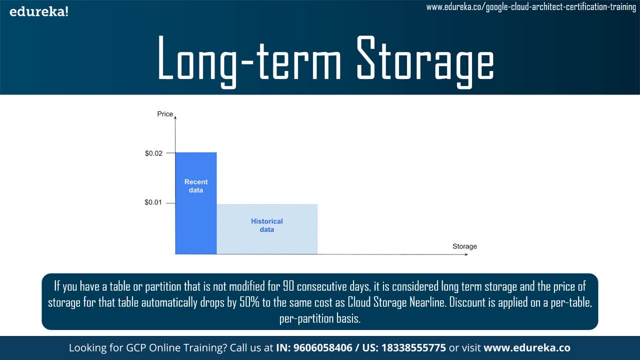 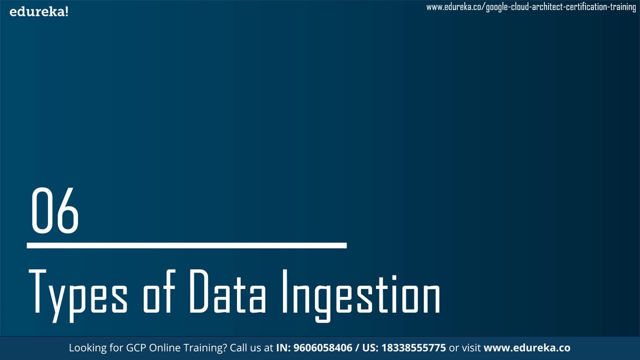 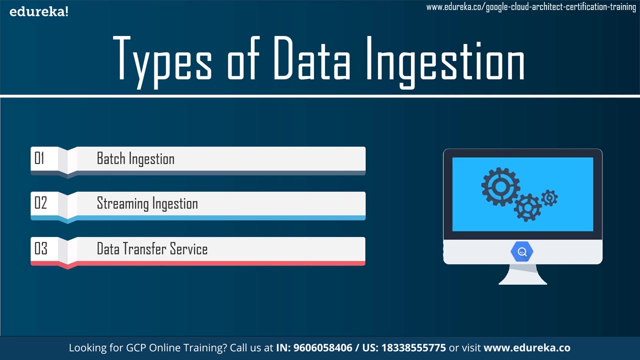 Since data remains in BigQuery, you can also query older data using the same interface, at the same cost level, with the same performance characteristics. Let us learn how to load or ingest data into BigQuery and analyze them. There are multiple ways to load data into BigQuery and depending on data sources, data 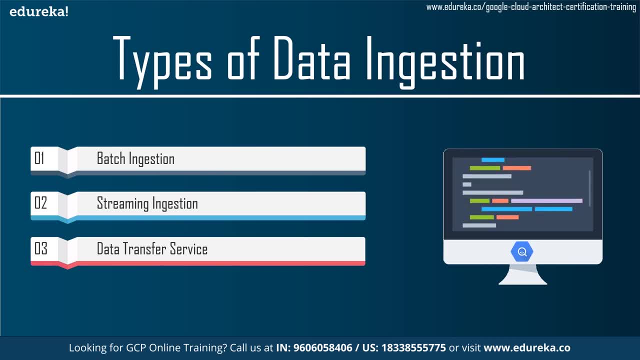 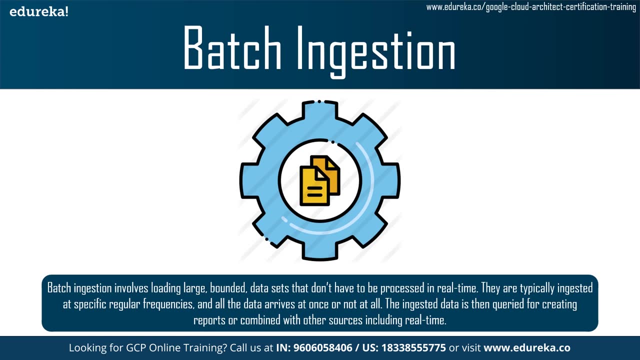 format, load method and use cases such as first one as batch injection. Second is streaming injection. Third one is data transfer service. So the first one is batch ingestion. So batch ingestion involves loading large boundary data sets that don't have to be processed. 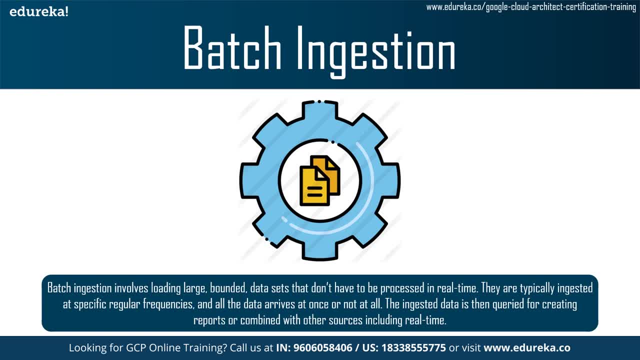 in real-time Now. they are typically ingested at a specific regular frequency and all the data arrives at once or not at all. The industry data is then queried for creating reports or combined with other sources, including real-time BigQuery batch loads. jobs are free. 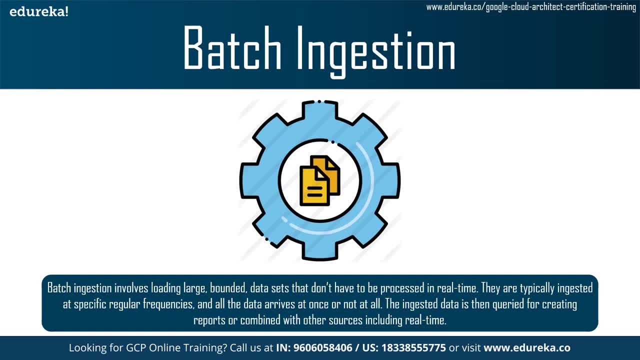 So you don't have to worry about that. You only pay for your storing and querying the data, but not for loading the data. For batch use cases, cloud storage is the recommended place to land incoming data. It is a durable, high-available and cost-effective object storage service. 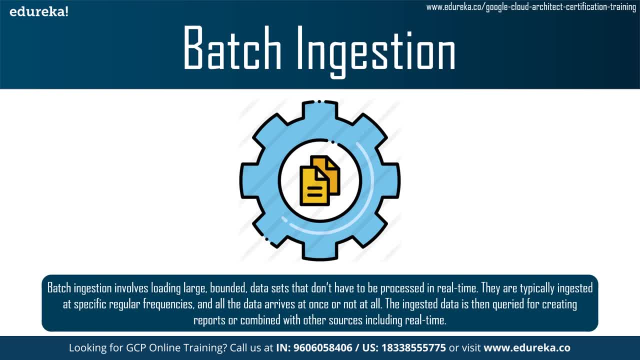 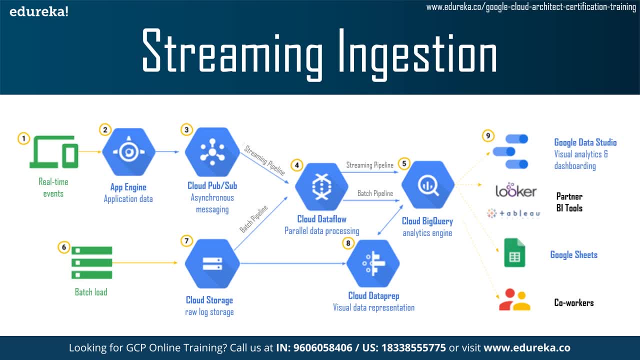 Loading from cloud storage to BigQuery supports multiple file formats like CSV, JSON, Avro and ORC. The second one is streaming ingestion. Streaming ingestion supports use cases that require analysis. It requires analyzing high volumes of continuously arriving data with near real-time dashboards. 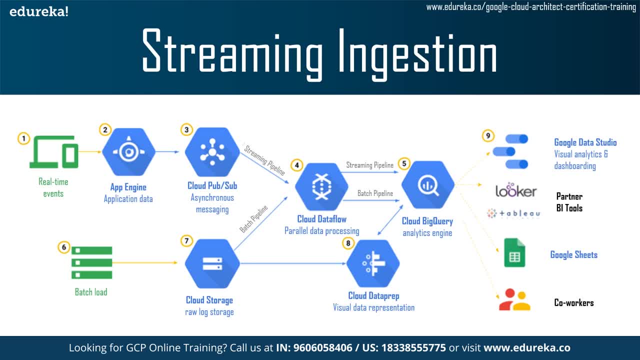 and queries. Tracking mobile app event is one example of its pattern. The app itself or the server supporting its backend could record user interaction to an event ingestion system, such as cloud pop-ups, and stream them into BigQuery using data pipeline tools such as Cloud Dataflow, or you can go serverless with cloud functions for low-volume. 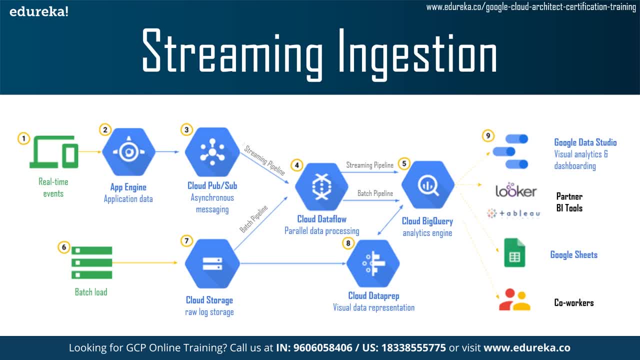 events. You can then analyze this data to determine overall trends, such as area of high interactions or problems, and monitor error condition in real-time. BigQuery streaming injections allow you to stream your data into BigQuery, one record at a time, by using the tableDataInsertAll method. 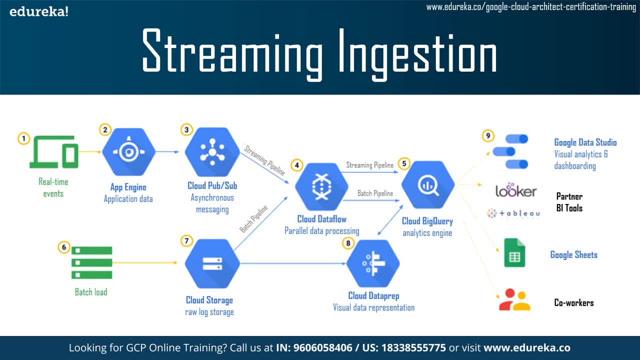 The API allows uncoordinated insert from multiple producers. Industry data is immediately available to query from the streaming buffer within a few seconds of the first streaming insert. It might take up to 90 minutes for data to be available for copy and export operation. 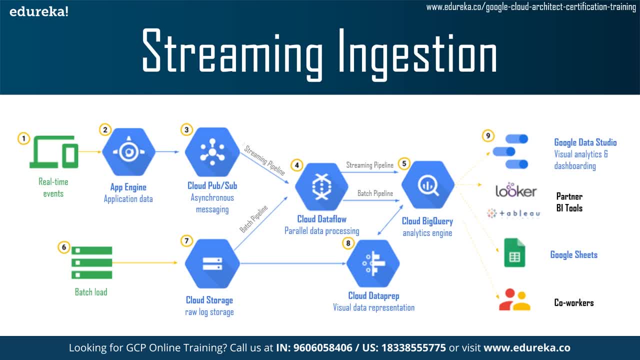 However, one of the common pattern to ingest real-time data on Google Cloud Platform is to read messages from cloud pop-up subtopic using Cloud Dataflow pipeline that run in a streaming mode and writes to BigQuery tables After the required processing is done. the best part with Cloud Dataflow pipeline is 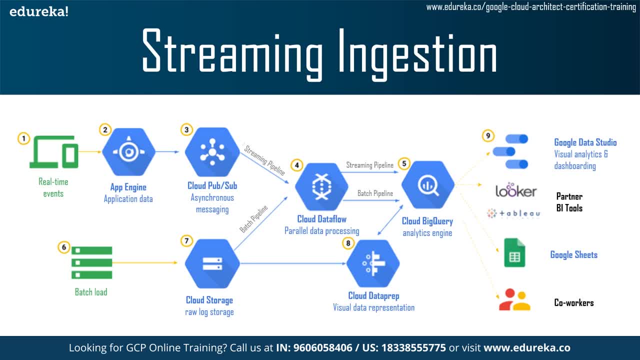 you can also use the same cloud for both streaming and batch processing. You can also use the same cloud for streaming and batch processing And Google will manage to work off starting, running and stopping compute resources to process your pipeline in parallel. The best part with Cloud Dataflow pipeline is you can also use the same code for both. 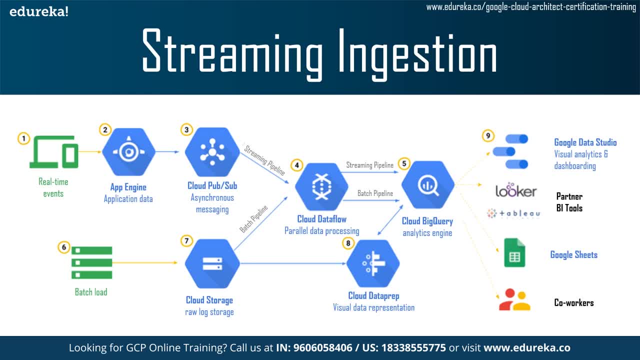 streaming and batch processing, And Google will manage to work for this reference architecture, which you can see here, is like Discover's use case in Master Trade. I hope you have understood till now, like Cloud Data Flowing, Cloud Pop-ups, How and What is. 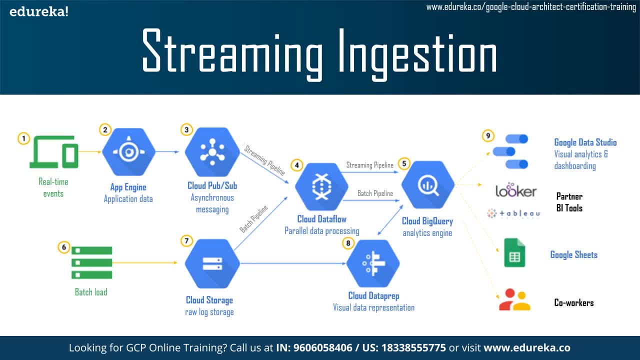 Cloud Storage. How does it works for making a cloud storage. How does it run? How does it run? What is Cloud Storage? By the way, Cloud Storage is an application to run on cloud through cloud data, So please note that you have option beyond Cloud Dataflow to stream data to BigQuery. 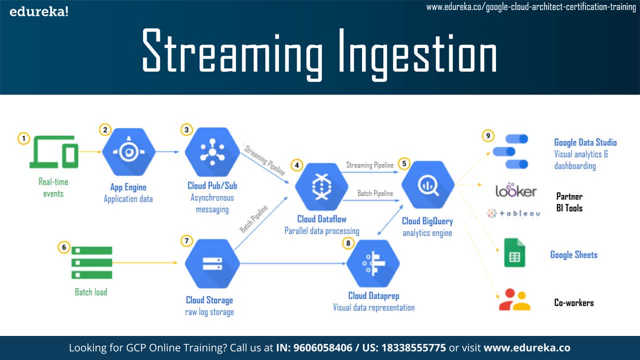 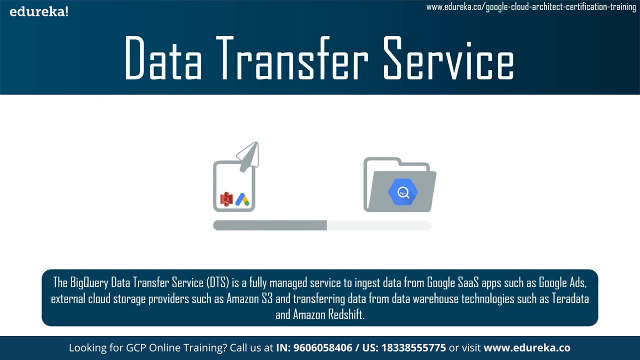 For example, you can write streaming pipeline in Parcher Spark and run on Hadoop cluster, such as Cloud Data Proc, using Apache Spark BigQuery connector. You can also call the streaming API in any client library to stream data into BigQuery. Now the third one is Data Transfer Service. 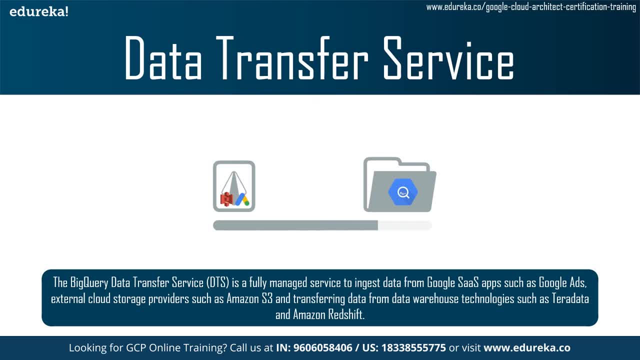 The BigQuery Data Transfer Service, GTS, is a fully managed service to ingest data from google software as service apps, such as google ads, external cloud storage provider such as amazon s3, and transferring data from the data warehouse technologies such as teradata and amazon redshift. 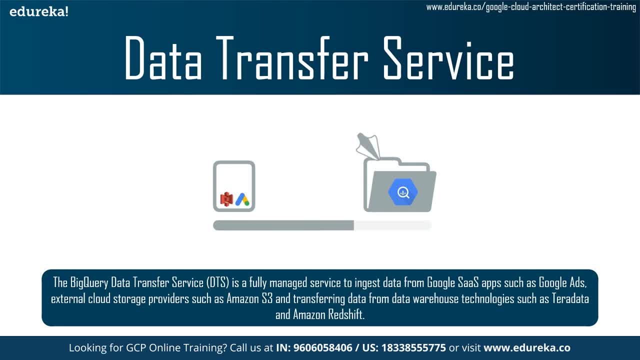 tts automates data movement into bigquery on a schedule and managed basis. now tts can be used for data backflips to recover from any outage or gaps. now think of data transfer service as an effortless data delivery service to import data from application to bigquery now let's now look at 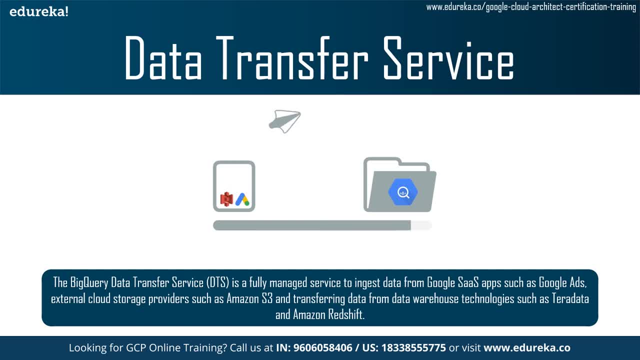 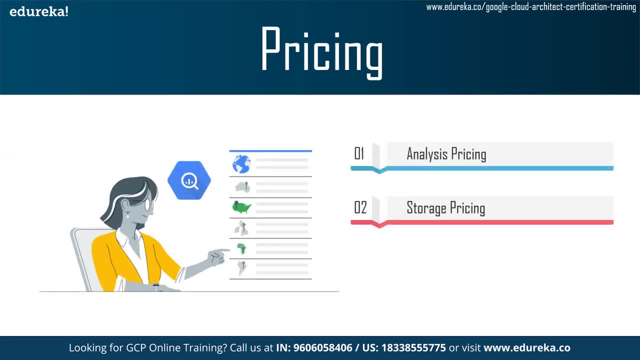 the pricing criteria and models of google bigquery. so bigquery pricing has two main components. so the first is analysis pricing, which is the cost to process queries, including xql queries, user defined function scripts and certain data manipulation languages and data definition language statement that scan tables. second is storage pricing. 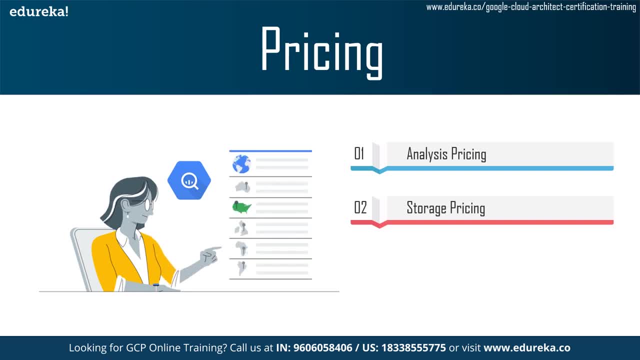 which is the cost to store data that you load into bigquery. each project that you create has a billing account attached to it and any charges incurred by bigquery jobs run in the projects are built to the attached billing account. the query storage charges are also built to the attached 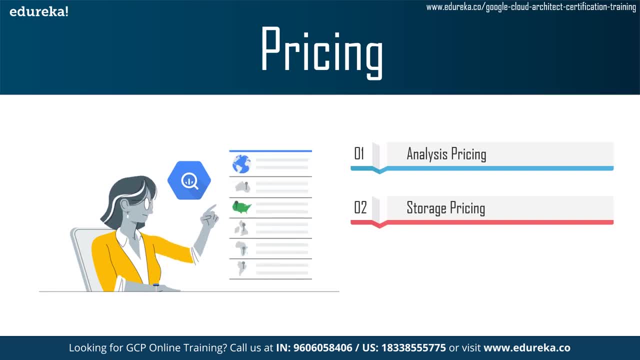 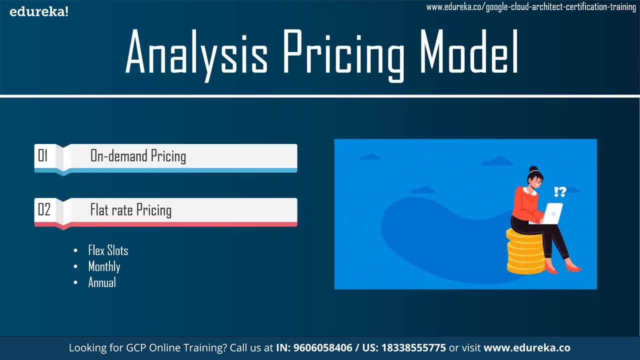 billing account. you can view bigquery costs and trends by using the cloud billing reports page in the cloud console. so let's discuss the first one, that is, analysis pricing model. bigquery offer a choice of two pricing models for running queries under this model, so the first one is the on-demand pricing. with this pricing, 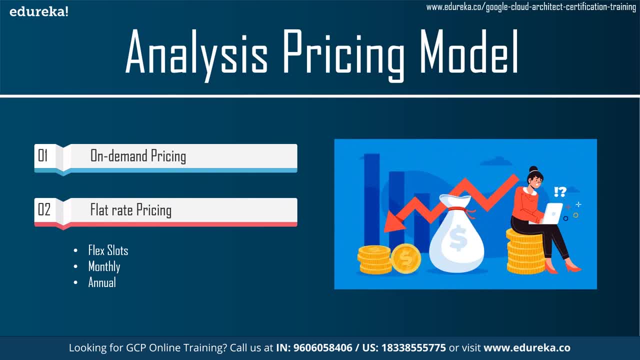 model, you are charged for the amount of bytes processed by each query. the first one terabyte of the query data process per month is free. second is flat rate pricing. now, with this pricing model, you can purchase slots, which are virtual cpus. now, when you buy slots, you are buying dedicated. 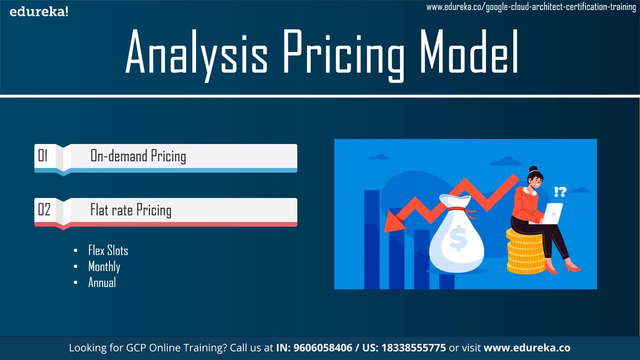 processing capacity that you can use to run queries. slots are available in the following rules, which are: которая um you can sell slots across multiple slots and use your own, your own connecting slots, or you can also purchase slots across multiple slots and you can use multiple slots to run a couple of tasks for each of your queries. so if you'd like to run, clientless slots, or you want to run your own ten day small contract slots, or you want to run your own non-client-only slots. a table will be set up in the description for the three terms sections in this method. so let's go ahead and go ahead and do that. as i have said in the previous video i used to use 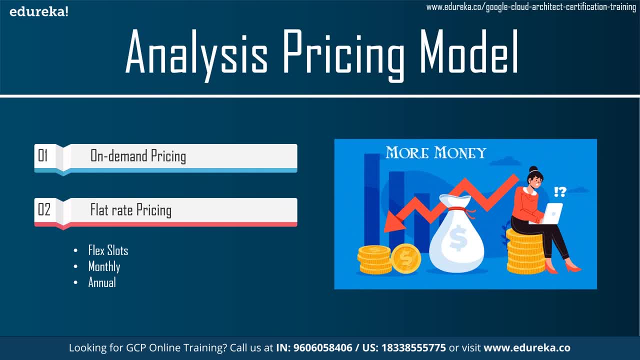 so performance can vary. Now, with flat rate pricing, your purchase guaranteed capacity with a discounted price for a longer term commitment. Let's briefly understand the first one, that is, on-demand analysis pricing. So by default, queries are built using the on-demand pricing model. 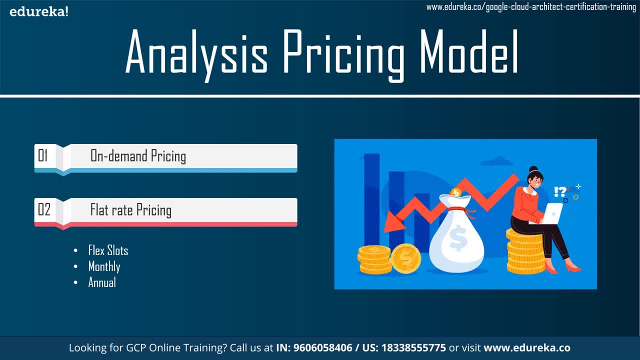 With the on-demand pricing, BigQuery charges for the number of bytes processed. You are charged for the number of files processed, whether the data is stored in BigQuery or in an external data source such as Cloud Storage Drive or Cloud Bigtable. On-demand pricing is based solely on usage. 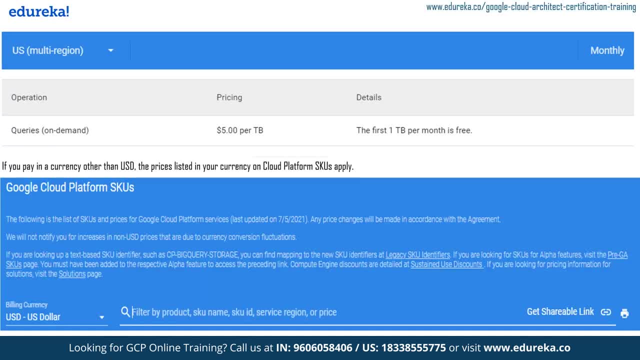 So this is how the on-demand pricing structure looks like. You can see, like queries on-demand are there, then they are charged for $5 per TB. The first one TB per month is free, and if you pay in a currency other than like US dollars, 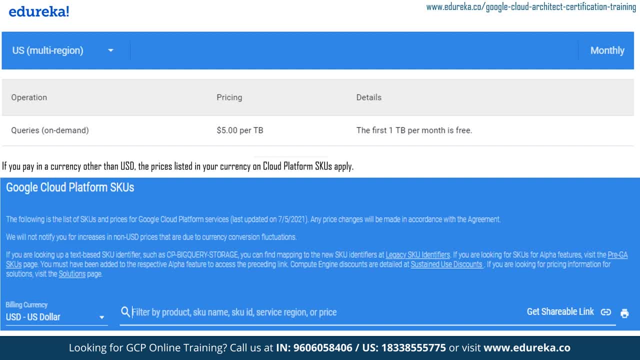 the prices listed in your currency. on cloud platform SKUs apply Like here. you can see the SKU is like how you need to choose your currency and you can filter it by product SKU name or the SKU IDs or service region or service. okay, Now let us discuss the second one briefly. 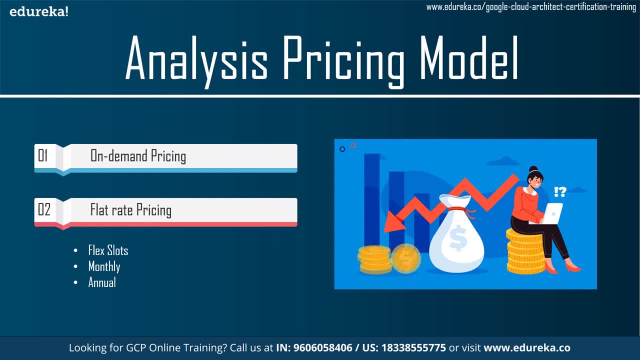 that is flat pricing, Now flat pricing. it is also available for high volume customer that prefer a stable monthly cost. Now BigQuery offers flat rate pricing for customer who prefer a stable cost for queries rather than paying the on-demand price per terabytes of data process. 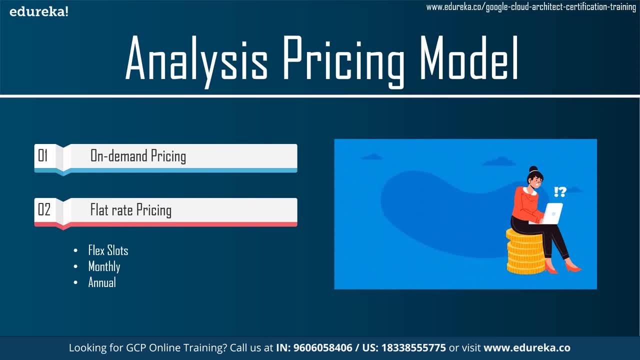 To enable flat rate pricing, use BigQuery reservation when you enrol in flat rate pricing Your purchase. dedicated query processing capacity measured in BigQuery slots. Your queries consume the capacity and you are not billed for bytes process If your capacity demands exceed your committed capacity. 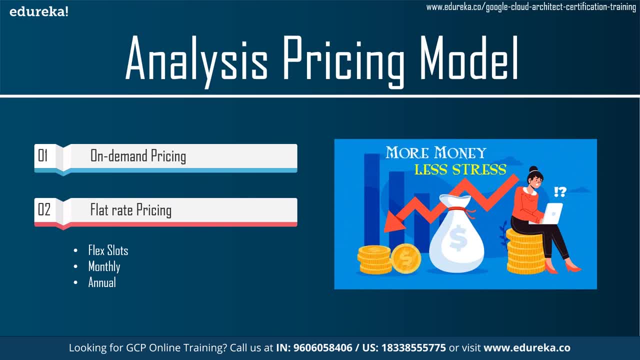 BigQuery will queue up slots and you will not be charged additional fees. So there are flex slots which have like short-term commitments. So flex slots are special commitment types, So commitment duration is only 60 seconds. Now you can see here. you can see here. 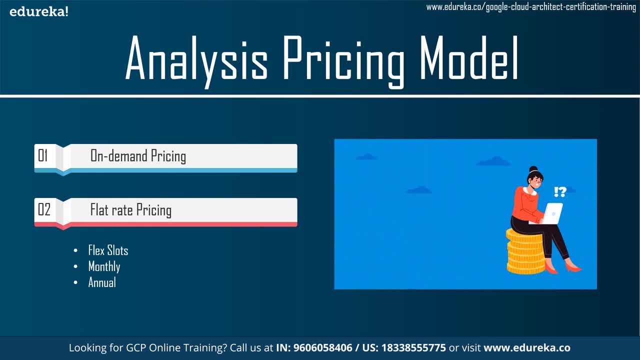 you can cancel flex slots anytime. thereafter, You are charged only for the second your commitment was deployed, So flex slots are subject to capacity availability. Now, when you attempt to purchase flex slots, success of this purchase is not guaranteed. However, once your commitment purchase is successful, 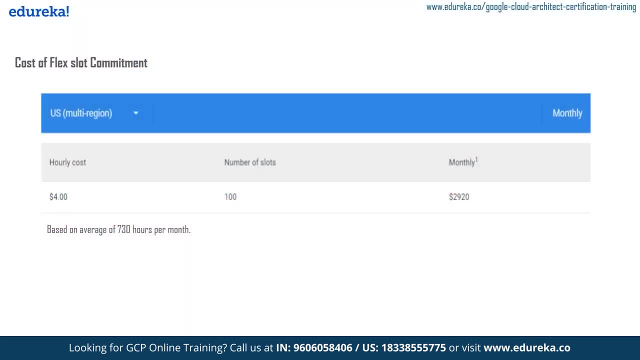 your capacity is guaranteed until you cancel it. The following table shows the cost of the flex slot commitment. Here you can see like how it's hourly cost. Now you can see like $4 for 100 slots and the monthly charges of 2,900.. 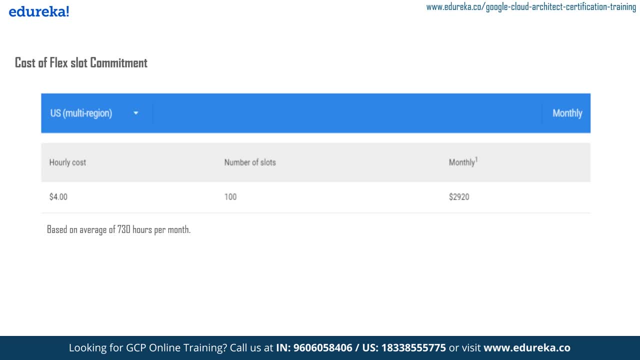 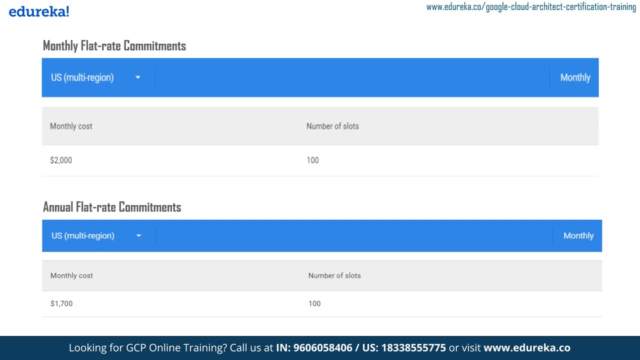 Based on average of 730 hours per month. Then there are monthly flat rate commitments. Now following table shows the cost of your monthly slots commitment. You can see $2,000 is given for 100 slots. Then there's also annual flat rate commitment. 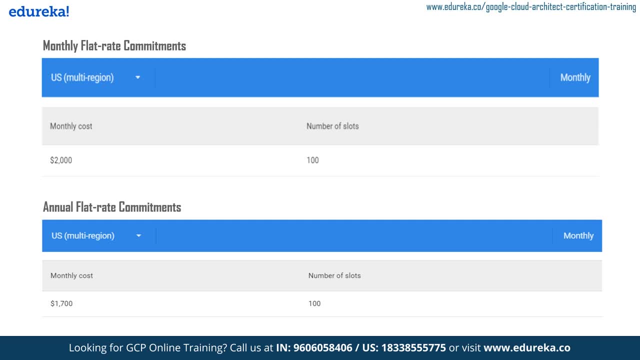 Now the following table you can see here, which shows the cost of your annual slot commitment. You can see the monthly cost of $1,700 for our numbers of 100 slots. All this is for us And it's for multi-region. 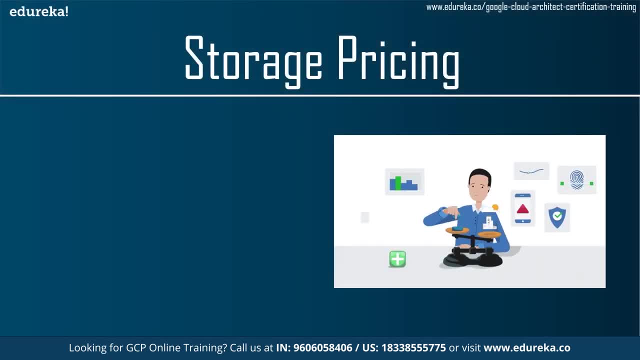 Let's move on to the second major pricing category, that is, storage pricing. So storage pricing is the cost to store data that you load into BigQuery. Now you pay for active storage and long-term storage. So active storage includes any table or table partition. 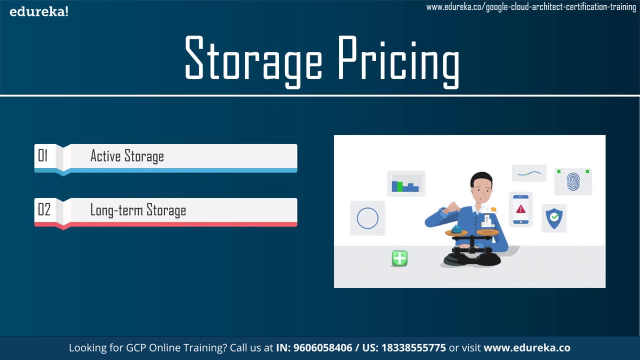 that has been modified in the last 90 days, And long-term storage includes any table or table partition that has not been modified for 90 consecutive days. So the cost for storage for that table automatically drops by approximately 50%. Now there is no difference in performance, durability. 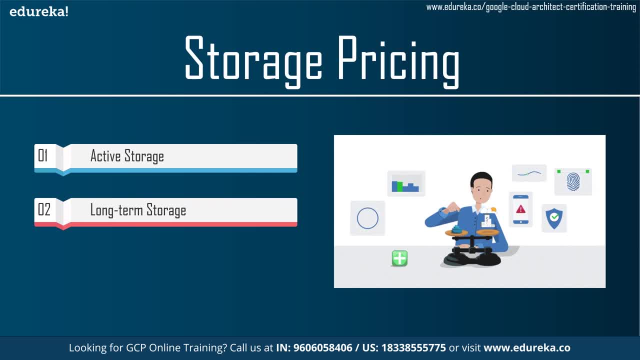 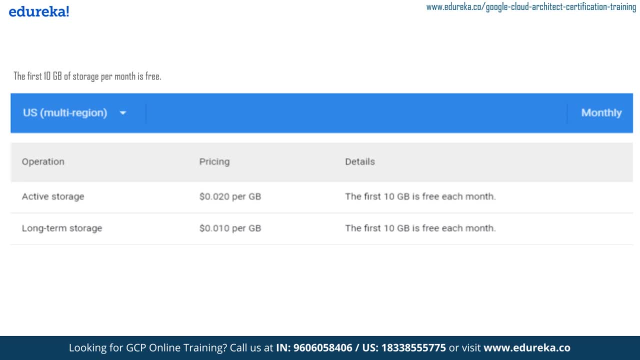 or availability between active and long-term storage. Here you can see: like the first 10 GB of storage per month is free and operation you can select like if it's active storage or long-term storage, Then pricing is given for like per GB pricing is given. 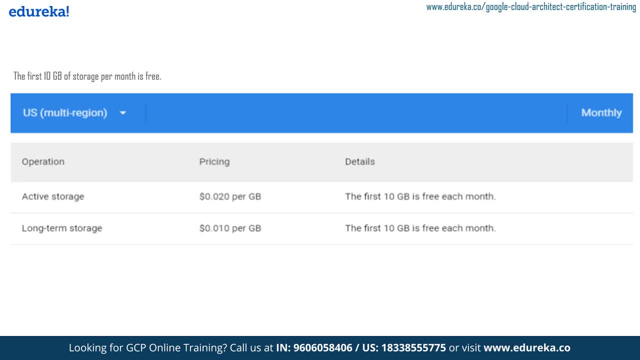 like you can see, for an access to it is $0.02 per GB And for long-term storage it is $0.010 per GB. So that's how you can see, like for a long-term, how the price is safe and in both of them, 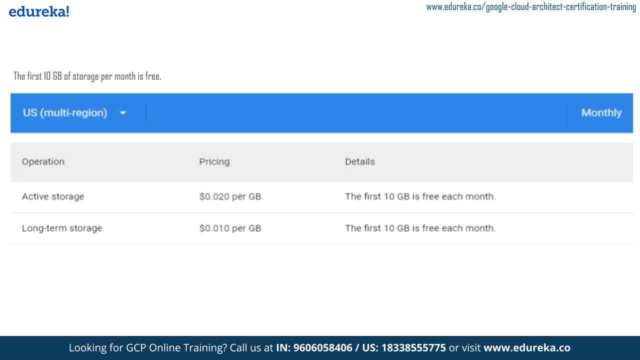 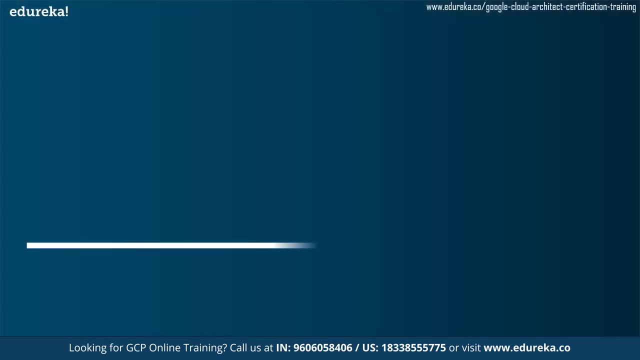 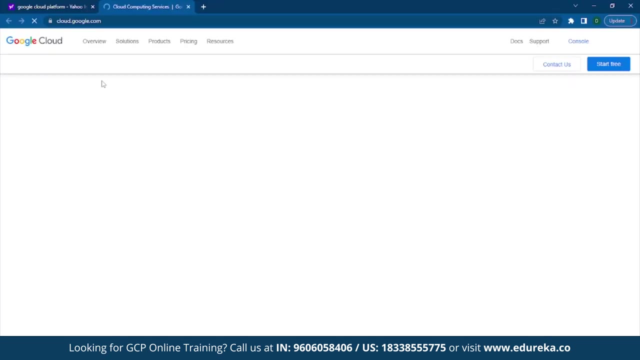 you can see like the first 10 GB in each month is free. Now that you have a theoretical and architectural understanding of Google BigQuery service, let's now see a practical implementation by trying a hands-on running it on Google Cloud Platform. So you can just go to Google Cloud Platform console. 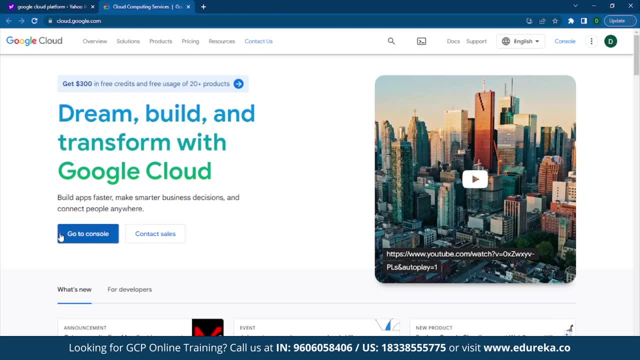 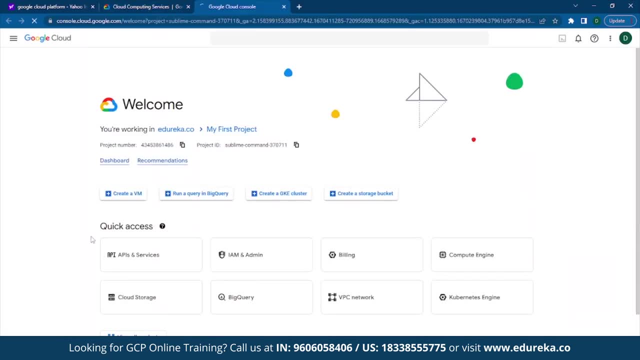 I already have a Google Cloud Platform account here, as you can see. here I can simply just go to console. So you don't have any account, so you can go ahead and create one. It's a very good platform to have your account on. 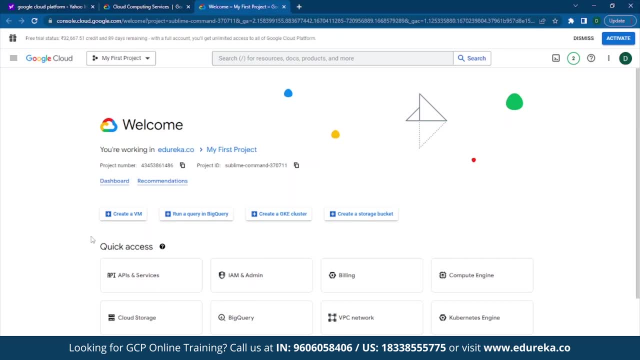 Also, you have to give your credit or debit card details. It will debit two rupees and it will also be refunded instantly and you will get 300 free credits for 90 days. Now you can use that credit for your own demo. I'm showing you. 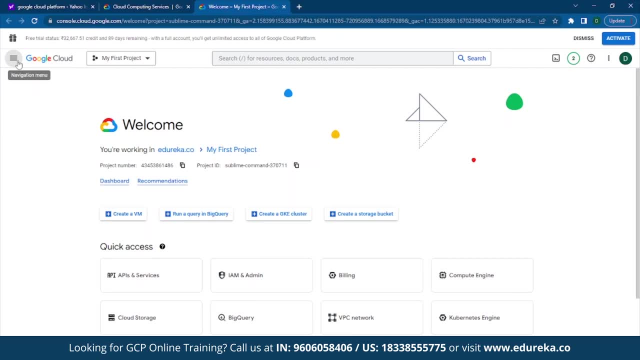 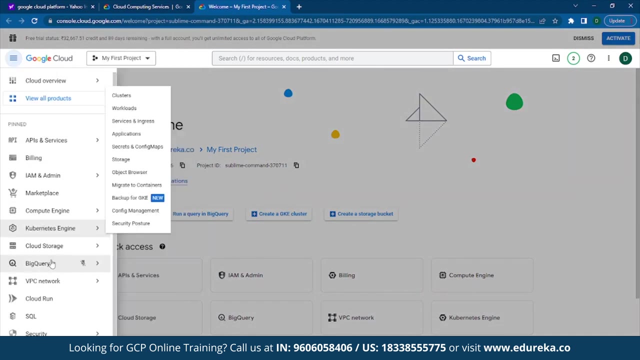 This demo you can go ahead and use for that purpose also and for using various other service on Google Cloud Platform. You can see the demo I'm going to show you doesn't require any cost. So let's start right ahead. We can go to BigQuery. under BigQuery, this is the one. 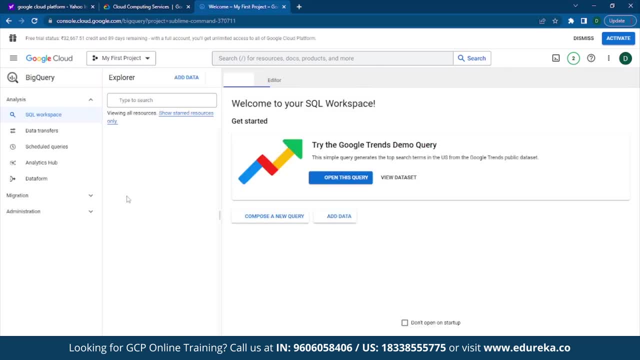 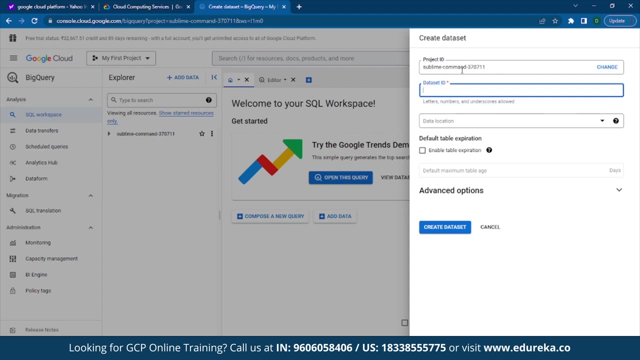 Just open it, create from start, So you can just simply click here And create data set. You have to give it a name, So your project ID is this- You can even change it if you want- And your data ID- This I'll simply write as data: demo. underscore demo. 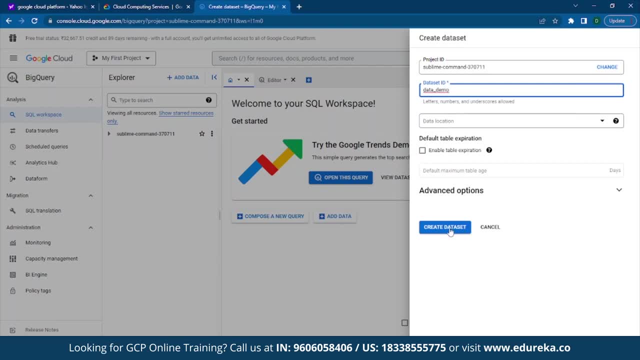 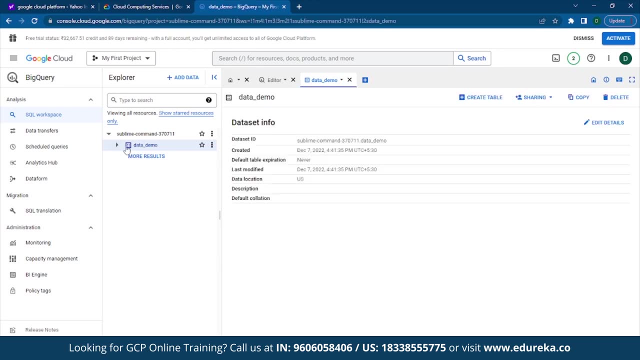 Location. put it to default Location. then we'll simply click on create data set And data set- you can see data demo here- And we simply create a table for that as well, for the data set we needed. So we then create a table. 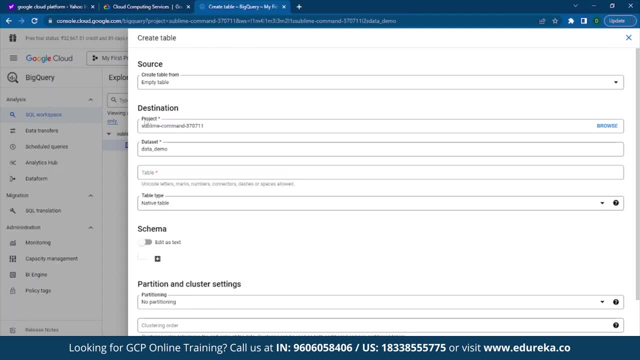 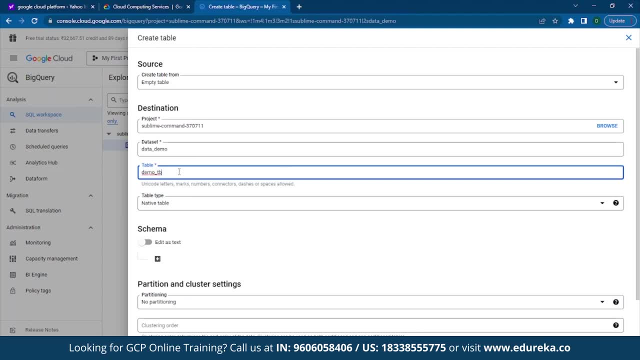 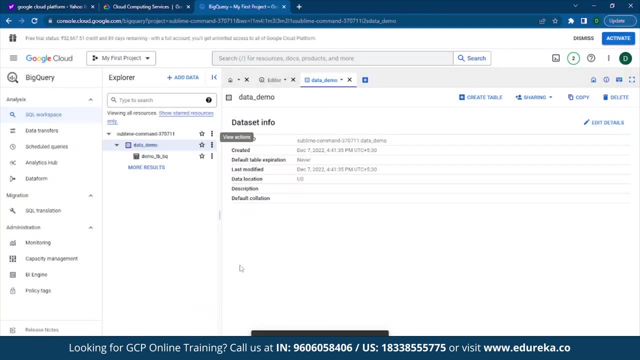 And you can name your table as demo DB underscore: BigQuery. So my table has been created. You can see. this is a table, This is the data set And this we have your data table. And this we have your data table. 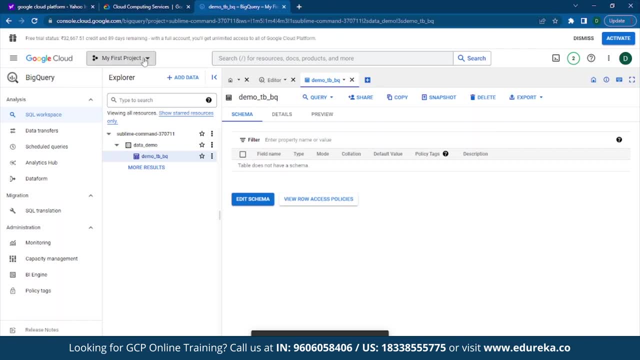 Now we can create a new project from here. Now we can create a new project from here. You can see here my first project. You can see here my first project, First project. So what you need to do is you can add data. 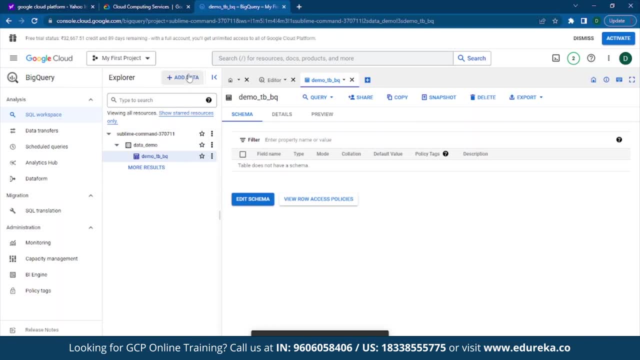 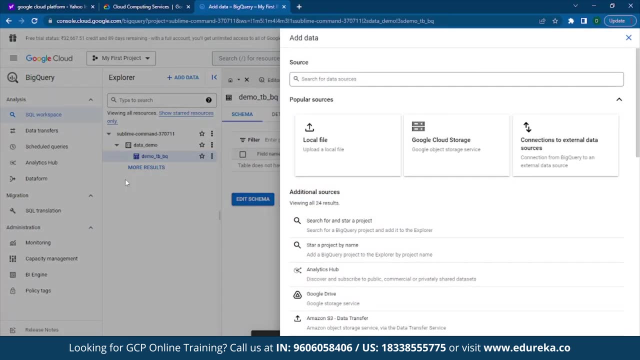 First project, First project, But it's here from a different place. So if I go here, Now what we are going to do after you press click on add data, Now what we are going to do today we are going to import a public data set. 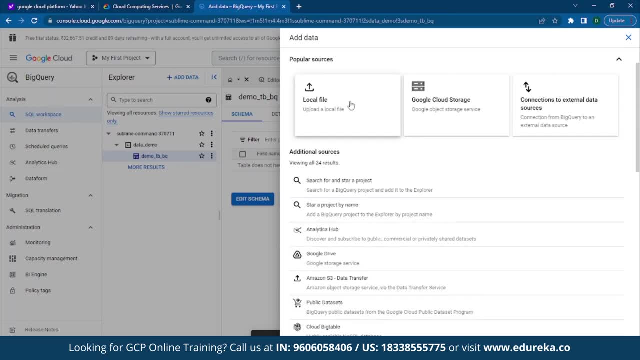 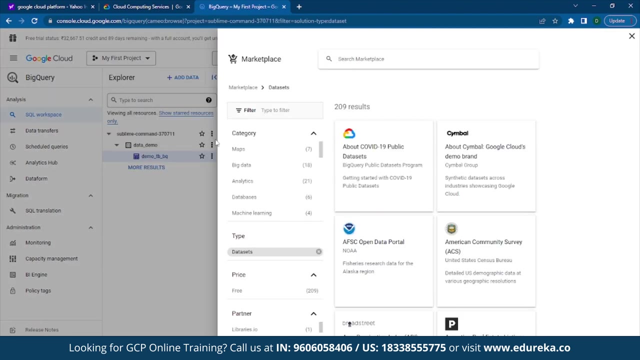 named stack overflow. You can simply import your file from the local file, or you can use your google cloud storage, or you can simply connect to an external data source. So in this demo I'll be showing you how I'll be using the public data set You can see. the latest one is 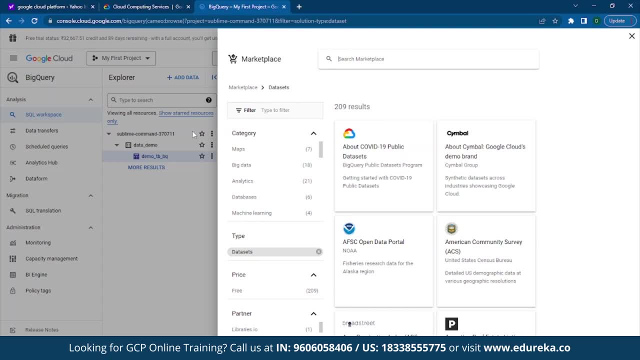 about the covet 19 public data set where you'll have all the information about the patients and how the cases are increasing and how the infected cases are increasing or if they are going down, whatever the analytic is there, regarding all the statistic and analytics, whatever is provided with. 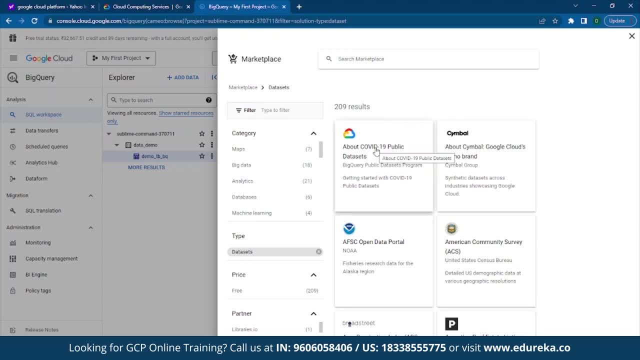 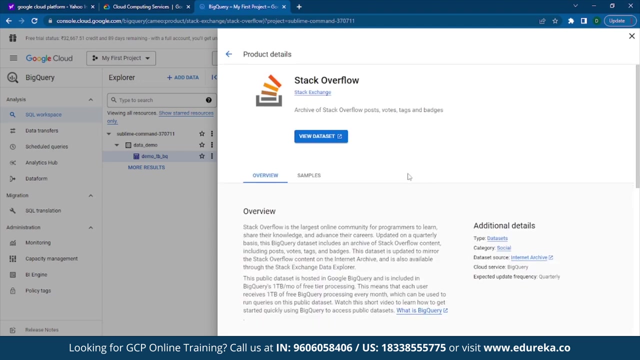 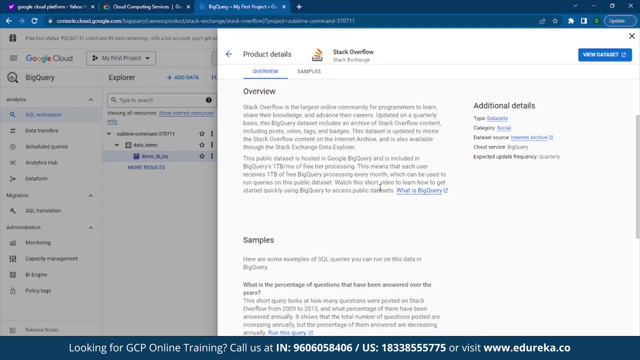 data of the covet 19. all those are provided here. in which state or which country? all those data are provided here. okay so, but we are going with the stack overflow, so we can simply click here and type stack overflow here. this, all the overview is given. like, what is stack overflow? it is the largest online community. 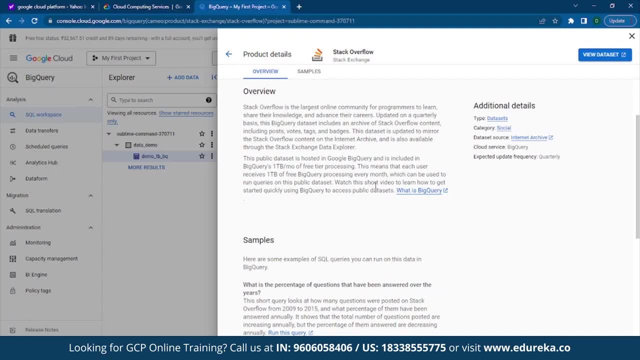 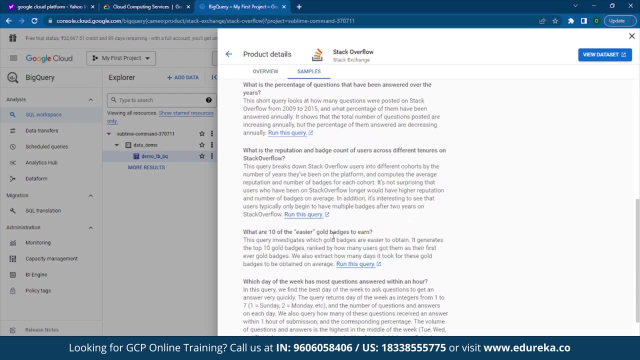 for learners to learn, share the knowledge and advance the credits. we know all these things. then they are sample, like here. there are many examples of sql queries. run this query on this sql queries as well. you can run these data. these are just a sample which are given. 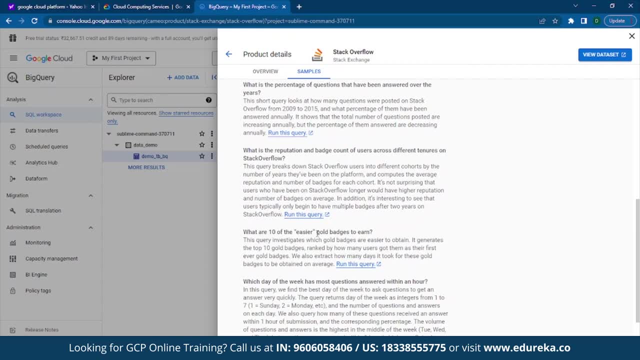 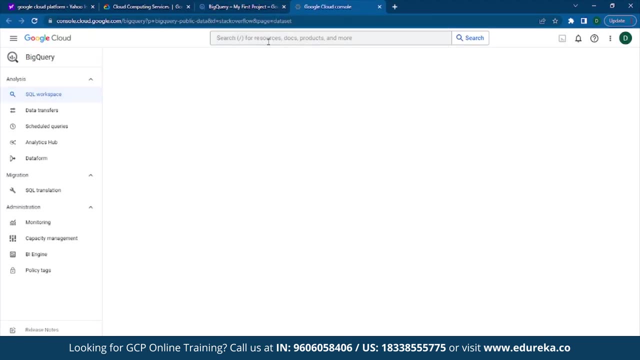 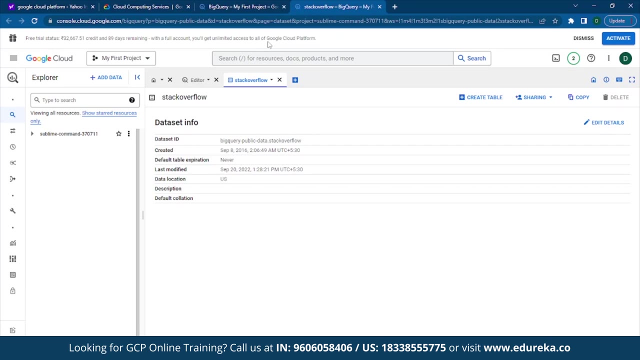 now the questions posted and the answer and all these things are there. now what we need to do is simply click on view data set. it will take us to another bigquery window, back to the query page. so yeah, so we are here now the data set has been imported. stack overflow: you can just click down. you can see here the 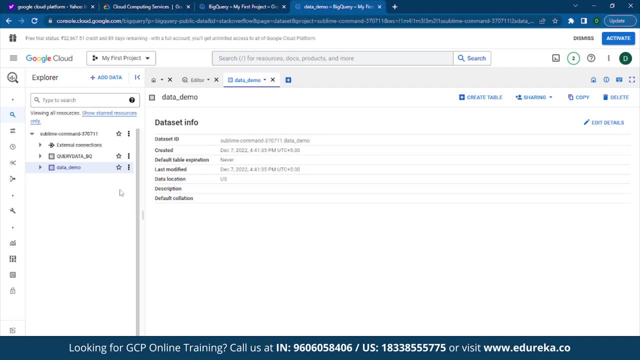 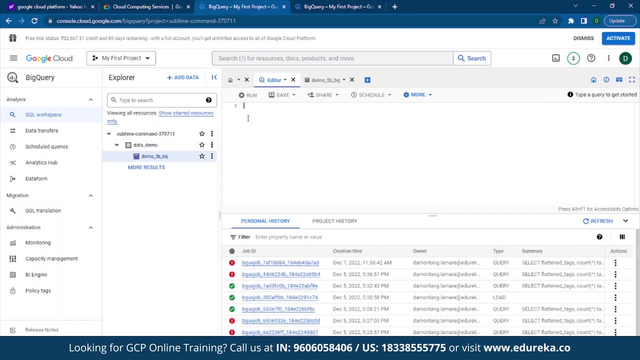 the table, and here is the table. so we have to query the table first. now what we have to do is we have to give the flatten text, so we have to select the flatten tax. so choose it from here, select tax, and then we can choose from attack counts to drag on the scope counts. so it's a select. 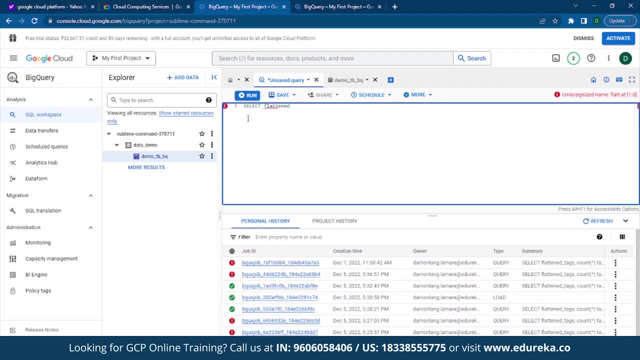 flatten, select and flatten underscore tax count and then you have select, so we have the spread of text tax from. okay, let's put it all this limit so we can remove it from from here. then select, split, then we put here the value as tax. 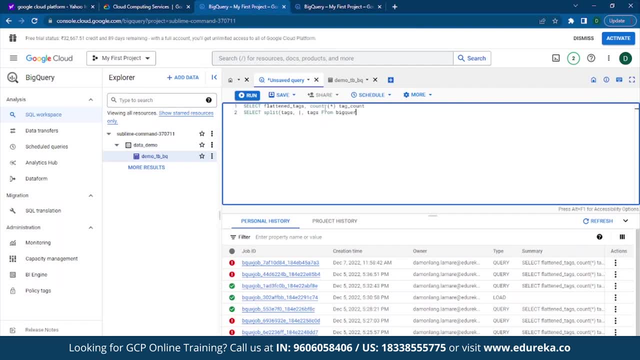 Now, from here we have to extract it, So like if there is any data column is given, so because we are finding the last ticket right. So which point from the creation date? okay, there is in this creation date, So we have to extract from here. 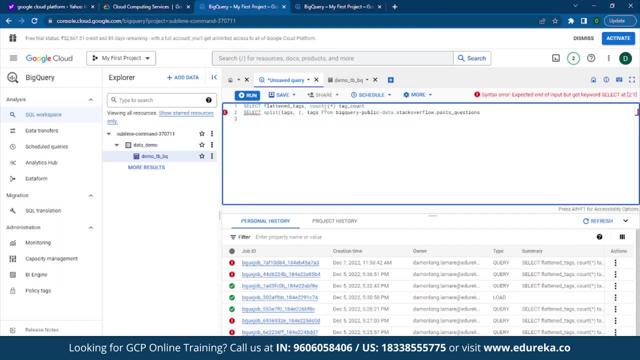 You want extract from the recent date here now we can just choose here here. so where then extract and extract then the year we'll have to join this. so put us cross, join and this we have the tax, Latin school tax. now you can group by flatten tax with a group by: 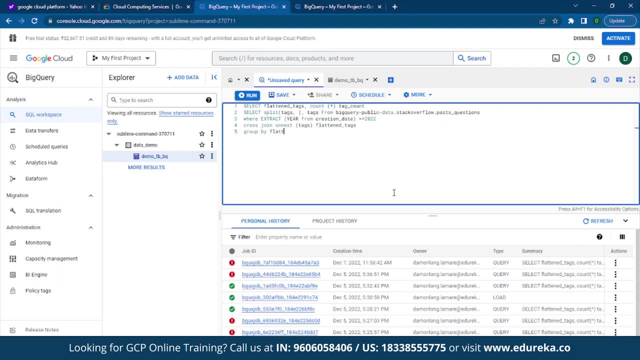 flatten tax and then we have an order to tackle. so order flatten underscore tax. then we have to order by that counts a in descending order. so order by tack and cone will be in descending order and we limit that to, since it's top 10. so limit there to 10. select split. 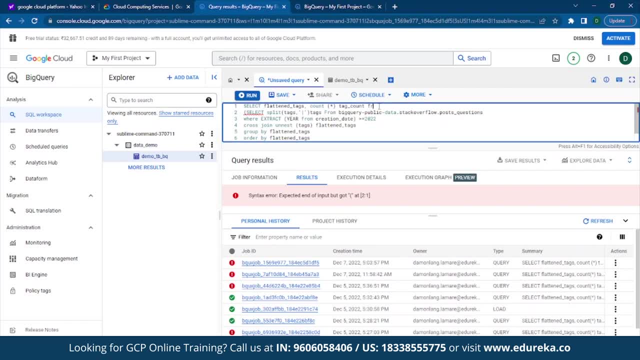 again, this shouldn't be from- was join, unless, okay, this should be for tax flatten, then tax synchro. okay, this seems fine. then simply click on. now it's done, so there's no more error you can. the process will take around 779.83 mb, which will run, so simply click on run. 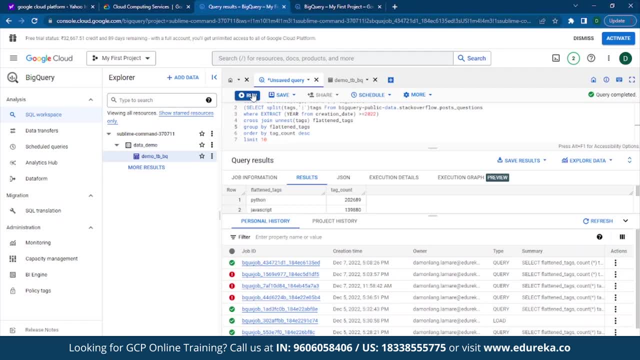 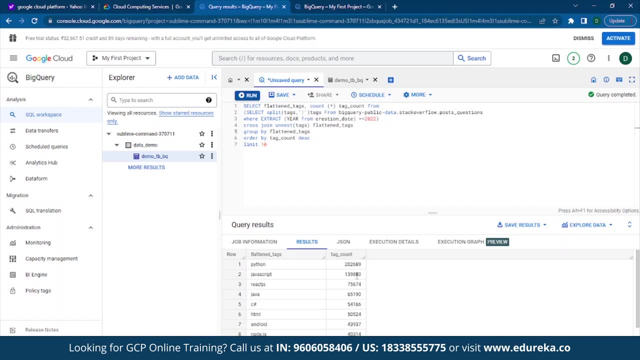 so this process should show it считable in eth Arabic in code or text i showed over here. we can just run the Sandy No Fill on us macro et cetera. to đây. we take a look at the process and we'll look at mine also, occasionally in a homogenidad way other. 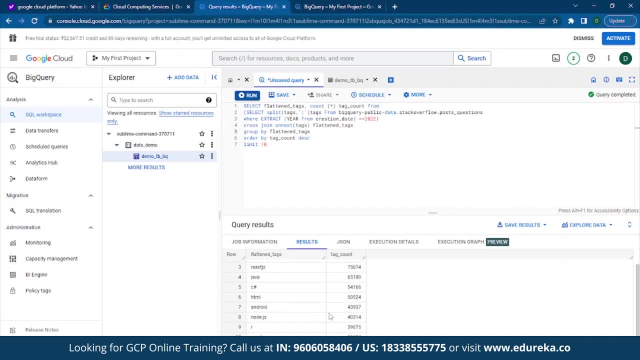 through today we're able to see that this method works here. so the first method is m1 and to execute aитm. so it is the default one, because we have more need for and plane and python is around two million to twenty six thousand two thousand six hundred eighty nine or. 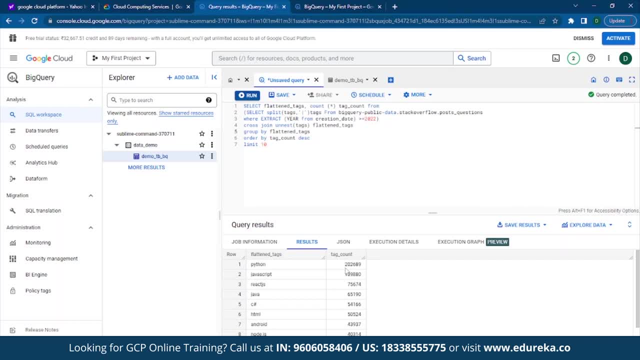 twenty thousand. so around python is around two lakhs twenty six, two lakhs two thousand six hundred and eighty nine counts. then you can see the json last decade. you can see their actions, like how many times they are searched. so we are successful here. now we can see the jobs. information is given. 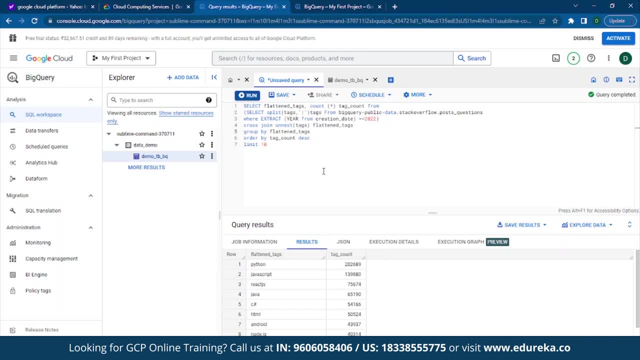 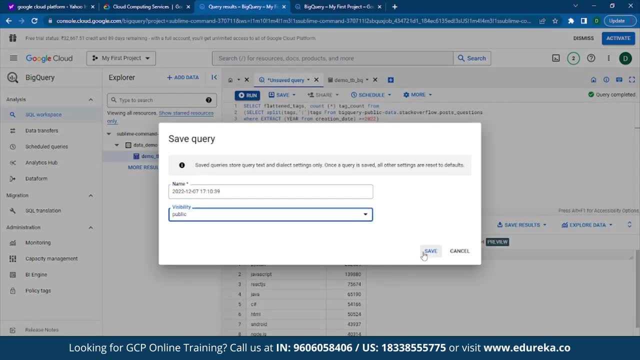 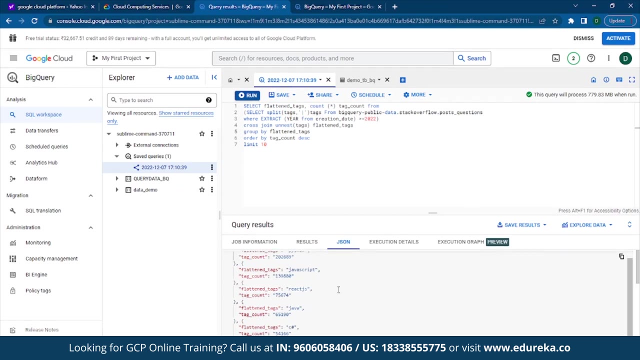 so what we can do is, when we just save this, we can simply save this save query, click this save and see it in json. you can see that counts here two lakhs. you can even see that is in json and you can see the panda: 35 684. 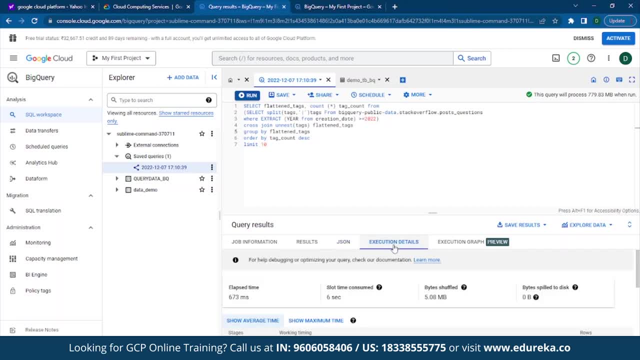 then we have here the execution details: how many times it took, like 673 milliseconds, and slot time consumed six seconds and the byte shuffle is for 5 mb and you can see for each weight as 230 milliseconds and the rows is like: uh, one hundreds 13 lakhs. it will reduce to record, reduced to 10.. 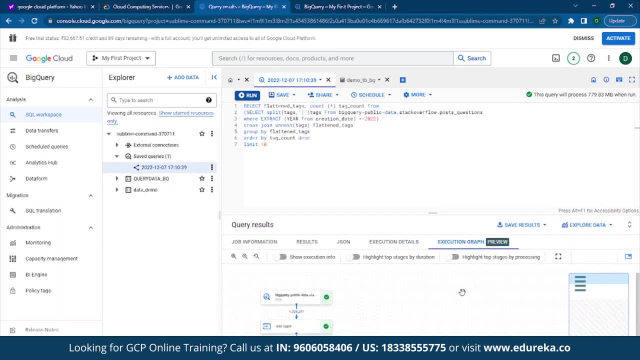 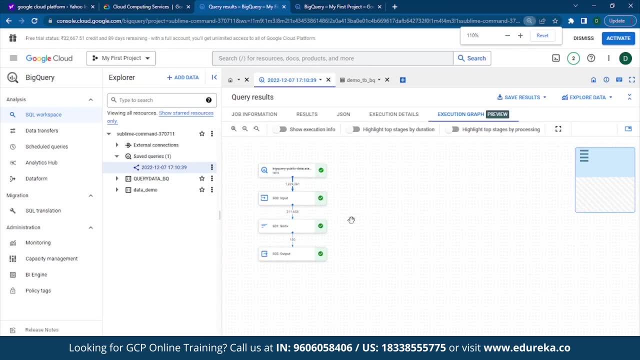 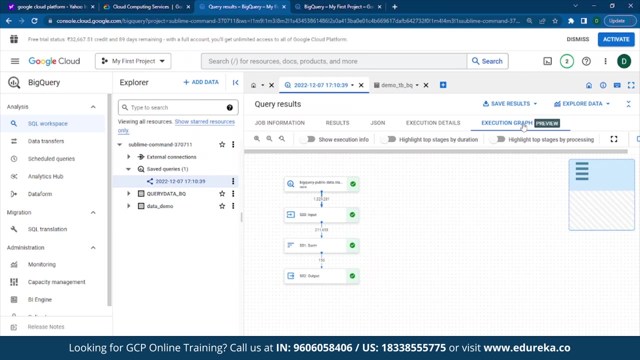 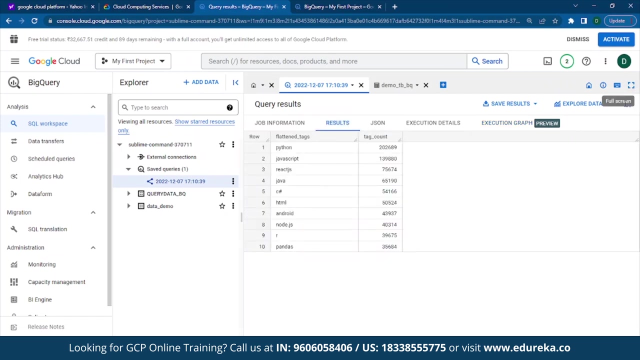 now if you can preview this, things a bit too small, just drag that upside so you can be able to see. you can see the input output from the sorting till the output of the view. data go back to the cell, as you can see. put this also down. you can also share this table. 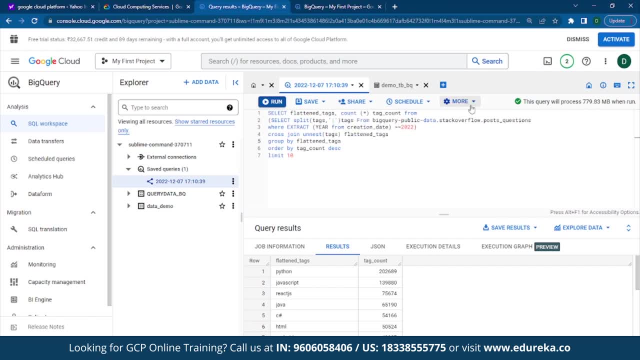 as you can see here, you can also share this table. well, you can copy the table and delete the table, or you can also export this table. you can also export, get the link and export the table, and you can also export it in google cloud storage. now, all these things you can do, and then you can have like save view also. 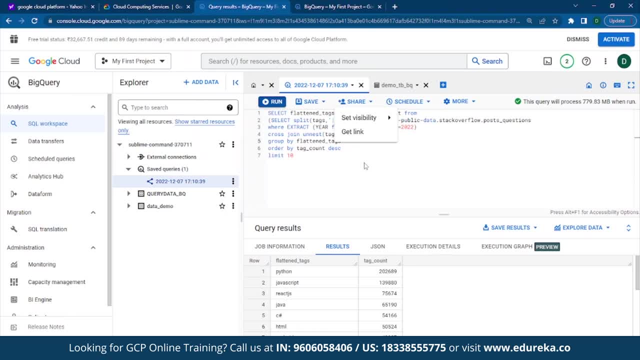 now, if you save this link, like it shows under view that how the table is working and the view you can explore this table also. third, very simple thing that i would show in the beginning. after this you can see here: explore with sheets, explore with local studio and with lab notebooks. save results. 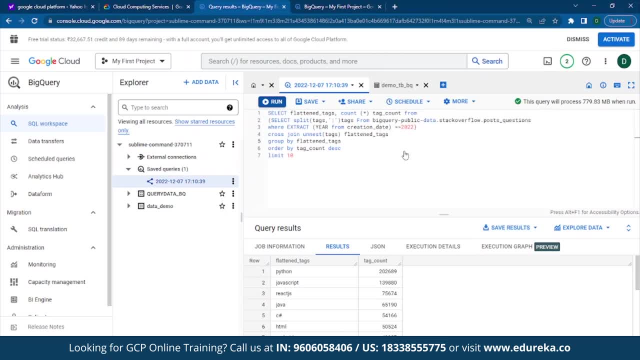 see, now you can share it through csv, json file or a big quiz table, so we'll save that so you won't explore. explore this time you can even schedule your query so you can create a new schedule query. but from this demo i'll just leave this for you and this is the thing that you can use if you wanted more dummy apps for your software to be used for rendering on. and many other things can also be done by creating custom files, because using your software won't. Patient's fala application works definitely scheduled. you can create a new schedule query, but from this demo i'll just leave it on atat 않는コ, so you can even schedule your query. you can even create a new schedule query, but from this demo i'll just leave it on another house. 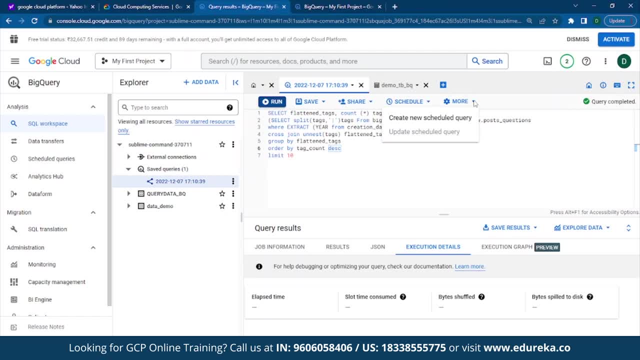 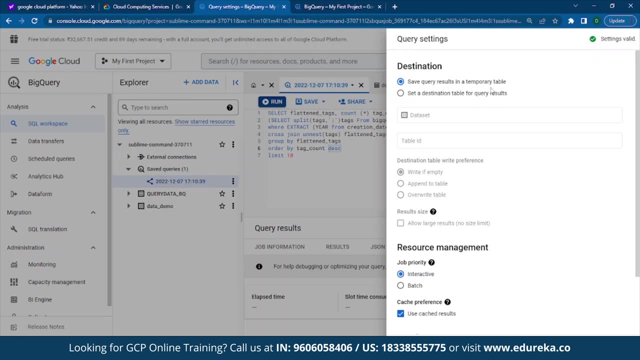 just leave it without creating a schedule and the next thing you need to do is if you go here, more you can go to, you can format your query or you can go to query settings. so query engines you can choose for what it's like cloud data, cloud data or a by query engine, and also if you are like querying. 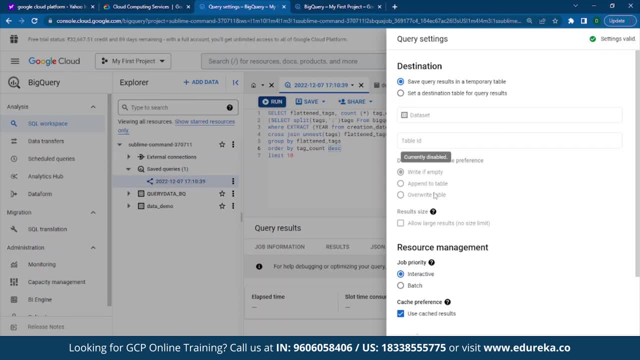 it and if you have forgot to save it, yeah, you can save here. it can get saved in the template tables. that temporary table, you can create it from here as well. you can see here all the things that have been there, like job priorities, destination tables. it can get safe in the template table. 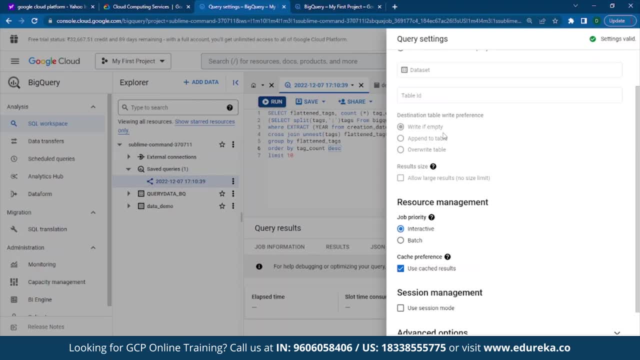 now you can create it from here. okay, now you can search it. all these things, like all these things that have been there, like the job priorities, then the system management: if you go to advanced option, see, as you can see data is encrypted or not, and then we have the sql dialects. 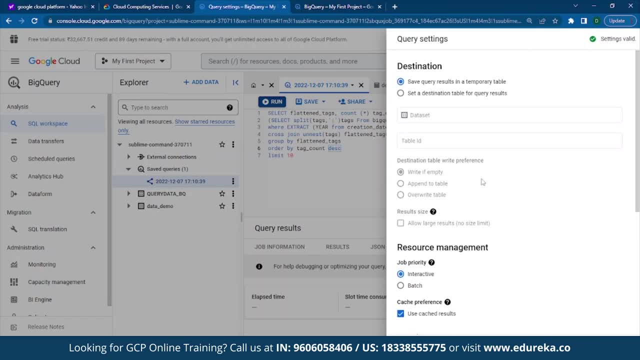 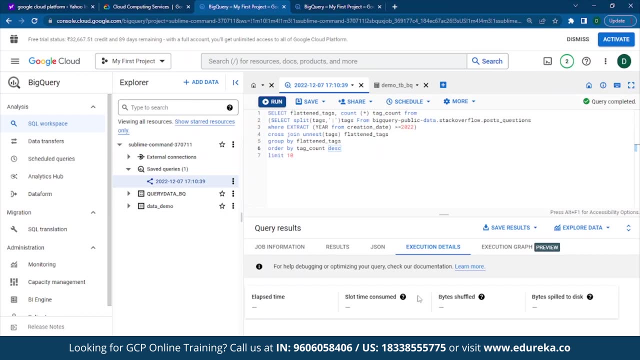 so the location? I have simply kept this as default with reference. now, all these things you can choose with the query settings, just canceling this. I hope you have understood it. now you can see how everything is provided at the dashboard. only every service doesn't take time. that's the thing about. 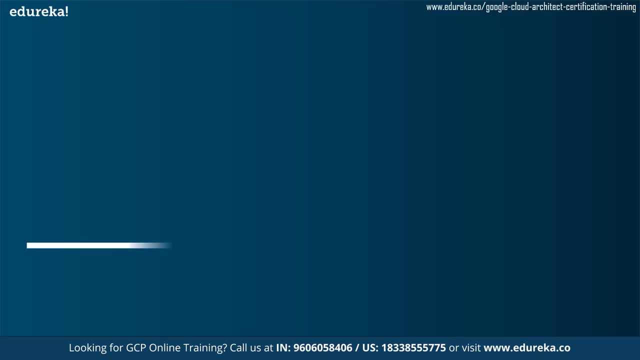 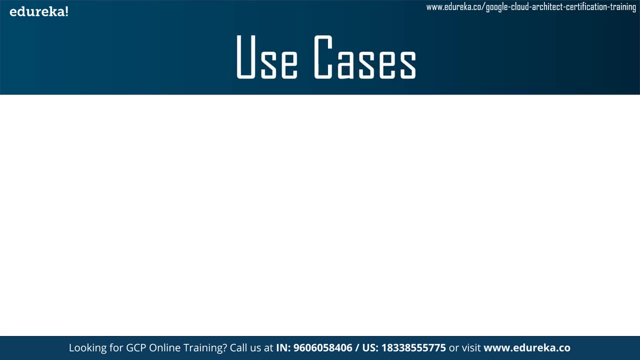 BigQuery that it is very fast. now let us understand some of the use cases for BigQuery. so the first one is migrating data warehouse to BigQuery so you can like solve for today, analytics demands and seamlessly scale your business by moving to google cloud, smart and data warehouse. 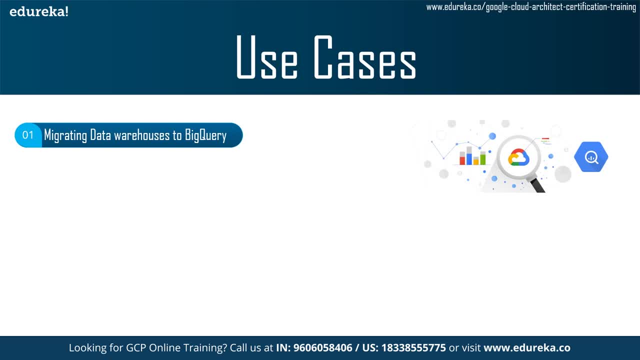 streamline. also you can streamline migrating path from netiza or oracle- redshift- there are data or snowflakes- to big queries and accelerate your times to insight. the second use case is predictive analytics. so predictive analytics helps you predict future outcomes more accurately and discover opportunities in your business. so the google smart analytics means BigQuery in google is smart and its 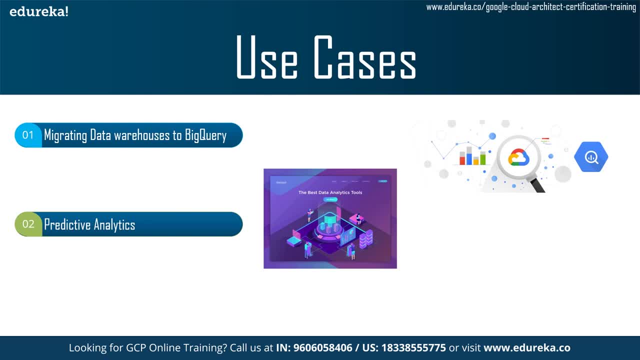 reference patterns are designed to reduce times to value for more common analytics use cases with small quotes and technical reference guides. you can like learn how BigQuery and BigQuery machine learning can help you build an e-commerce recommendation system, but also like predict customers and lifetime value and design propensity to purchase solutions. also, you can bring any data into big. 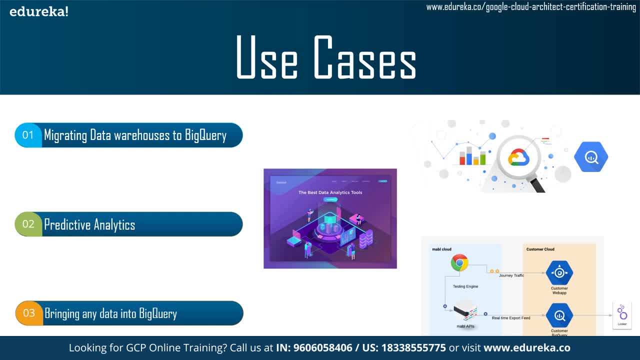 query. make analytics easier by bringing together data from multiple sources in BigQuery for seamless analysis. now you can upload files from local source, google drives or cloud storage bucket takes advantage of BigQuery data transfer service now data fusion plugins. or, we can like, leverage on google, industry leading data integration partnership. now you have a lot of data to use in your business. 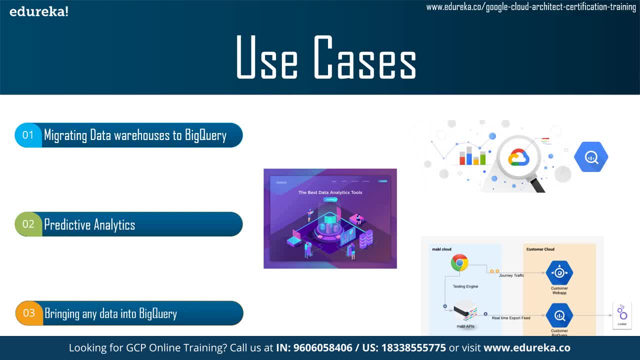 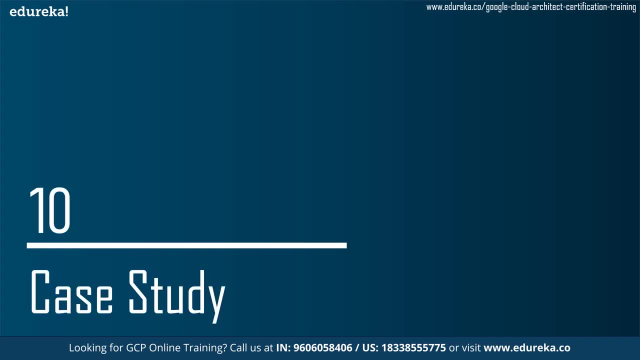 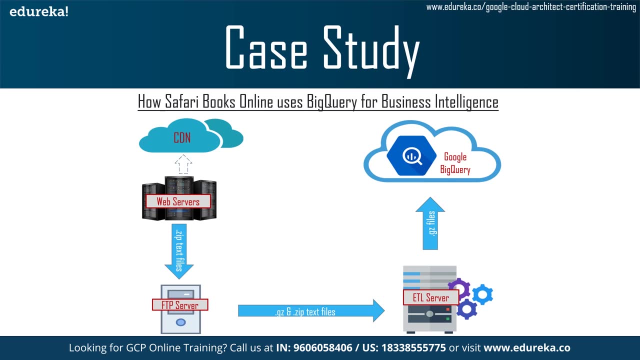 so if you don't have pinpoint data, so you cannot bring specific optimize data. that uses Haddock API. so let's now do the data, Alice. so let's now see the case study for Google BigQuery. its definitely topic we are discussing. then you will wrap up. we can see here: we have the safari book online, which uses BigQuery to solve a few key. 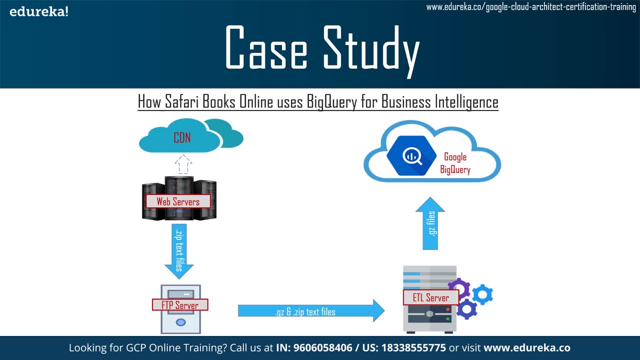 queries to answer specific business questions. so all these things we will understand step by step. so what they did is they choose bigquery over other technologies because of the speed of querying using a familiar sql like language and the lack of required maintenance. so safari books online has a large and diverse customer base constantly searching for accessing a growing library of over. 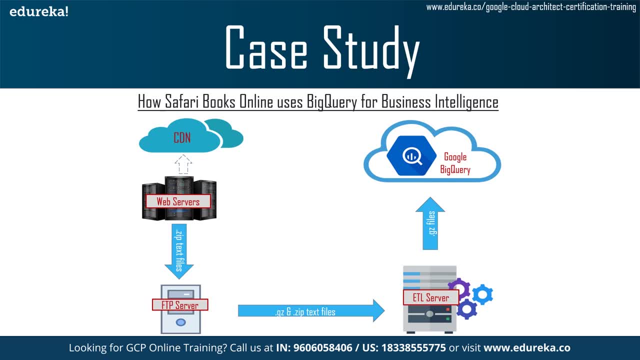 30 000 books and videos from an increasing array of desktops and mobile device. this activity streams contain powerful knowledge which we can use to improve our services and increase profitability. locked up in the mountain of usage data trends, such as the top users, top titles and 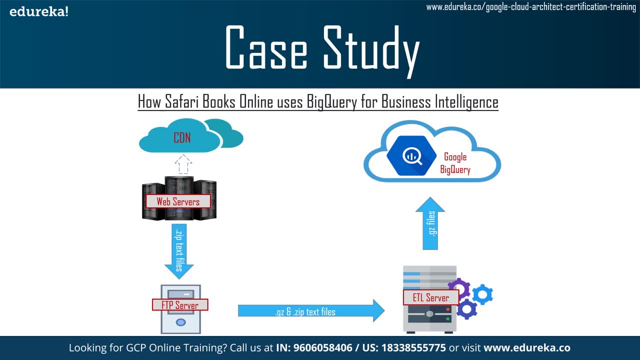 correcting the dots for sales inquiries. safari usage data was much too massive to query online entirely with the previous tool. said analysis could be done with the third-party web analytics tools such as the home nature, but those tools lacks the ability to query and explore record levels data in real time. 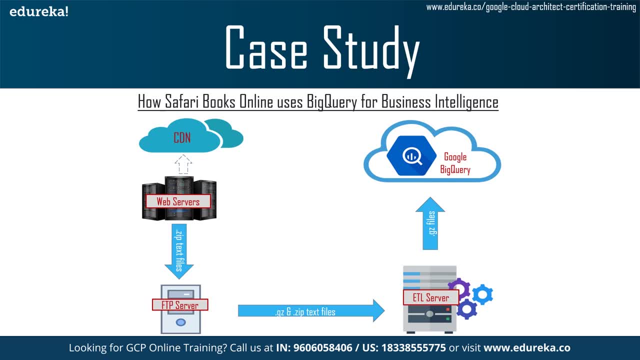 in addition, they didn't have a great background for developing visualization sql, like pairing had to be done on a smaller chunks of data and was labor and 10 seconds slow. now they were impatient, waiting for my sql queries to finish and were often in doubts as to like whether or not they 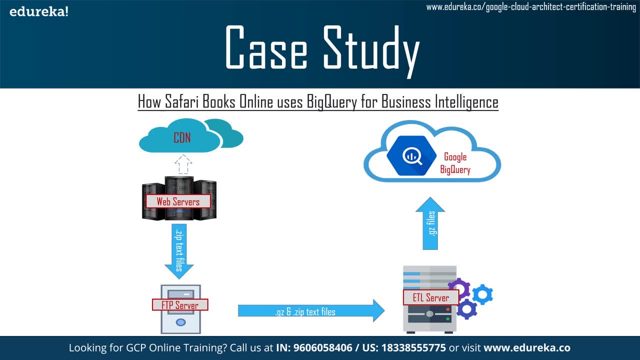 should finish at all. once you reach a database client time out of 10 minutes, you are not in the realm of not being able to do like ad hoc analysis. answering often operational questions can be like a time sensitive. so speed is important, of course, it's very important. so safari organization has actually like played. 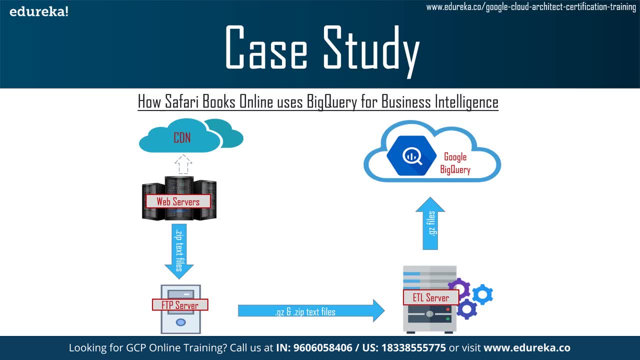 with hadoop, but it proved to take a lot of resources to maintain so they ended up putting it on the back burner for further projects. then they learn about the google bigquery through a video from google inputs and output determined it seems perfect for their use case, so they decided to try it out. so first step is like you can see here in this diagram. 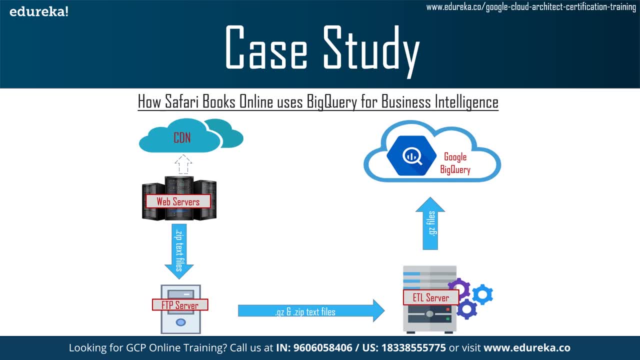 this tells you how safari gets the data into bigquery. so, no matter what database platform you use, the extract transform load setup can be a challenging depending on your data sources. bigquery is no exception. i will say then: this diagram shows an overview of how the data flows through the landing and etl server leading up to bigquery, the usage. 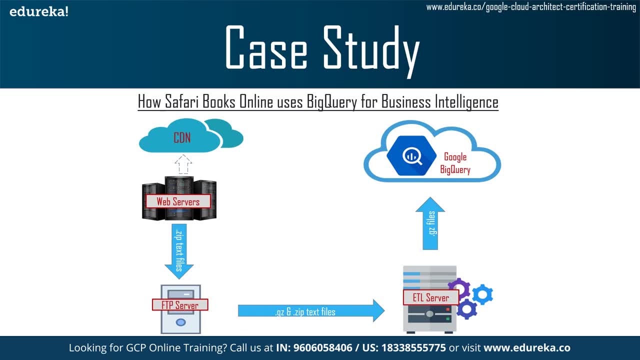 data comes from content delivery network in the cdn and web application server logs. this data was packed into time-based batch chunks, automatically copied into a landing directory. it needed some transformation to load the data into the bigquery server so you can see here that the data is now. 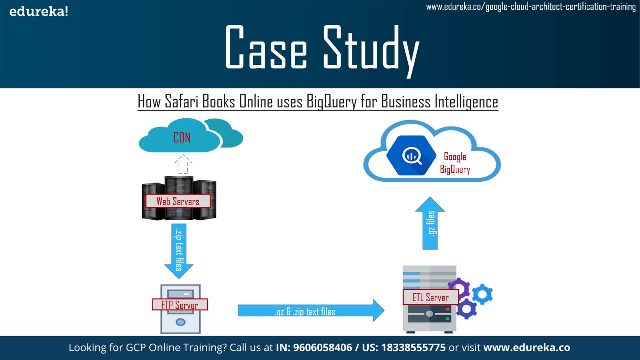 loaded into bigquery in a format where we can get the most use out of it. here are the basic steps safari went through. so it got a list of all sources files that have previously loaded into bigquery. then validate the list of sources files waiting to be loaded into. 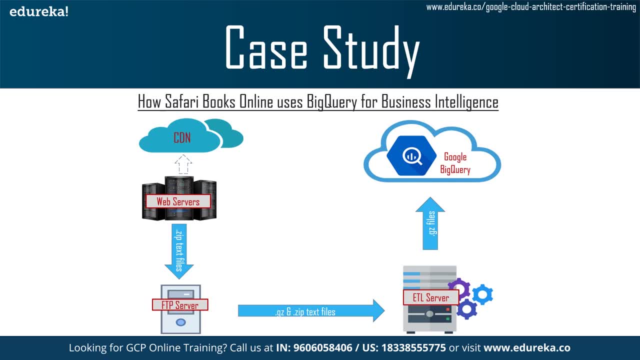 bigquery, then transform the files and copy the file into bigquery cloud storage, then load the files into bigquery and finally use the data once it is in bigquery. so bigquery proves to be a good platform for dashboard data and offers the capability to load the 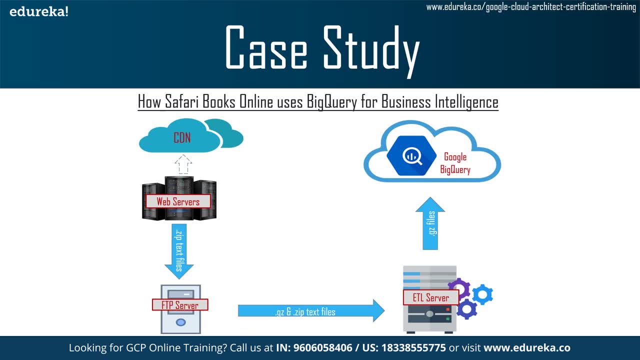 data in the dashboard further with big data query browser and offer the capability of drilling into the data in the dashboard further with bigquery browser base ui for adopt analysis. so here you can see like it's a dashboard used internally by safari operation teams to monitor top user if 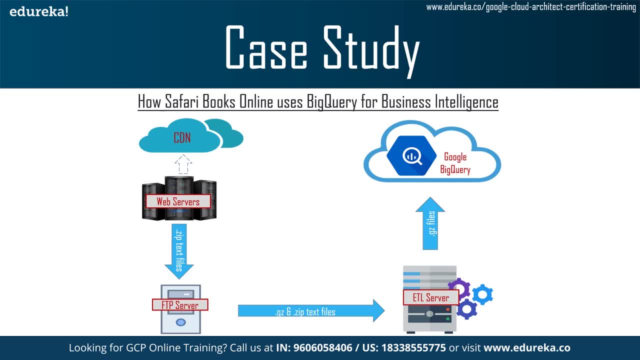 anything raises any questions. you can get more information about a user title and ip address by querying with the bigquery browser tools. now you can see here the dashboard safari uses internally to keep an eye of the trending top titles. again, if anything raises any questions in the dashboard, bigquery can answer them. 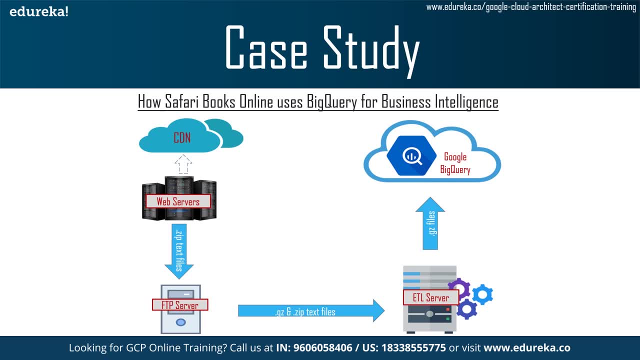 for you. now the data is fed to this dashboard by an intermediary schedule, jobs, which is executed via the script queries. now bigquery is with the bigquery line tools, gets the result in json and then contact some other web service to get more information, which is not stored. 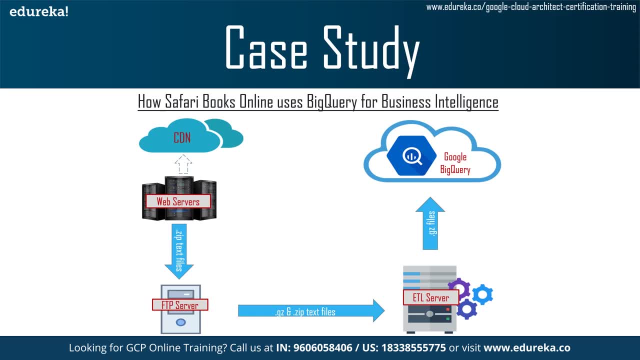 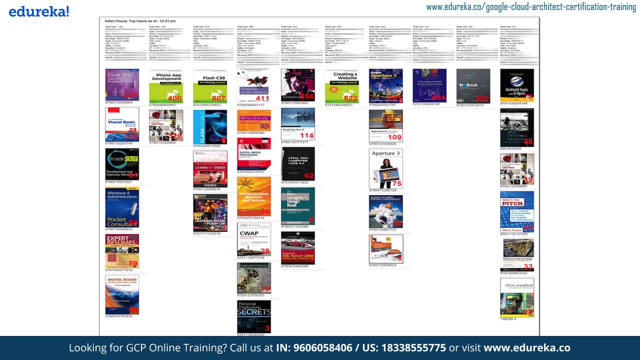 in bigquery, such as the user data and the book thumbnails image, then it's all match up and presented in the dashboard. this is a good pattern, as you won't want to query bigquery every time the dashboard was loaded, as it will get expensive. it is best to do. 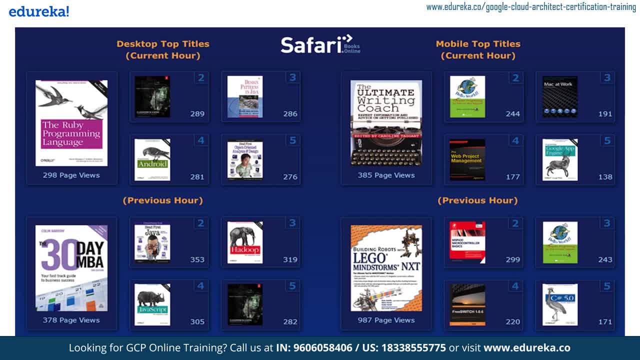 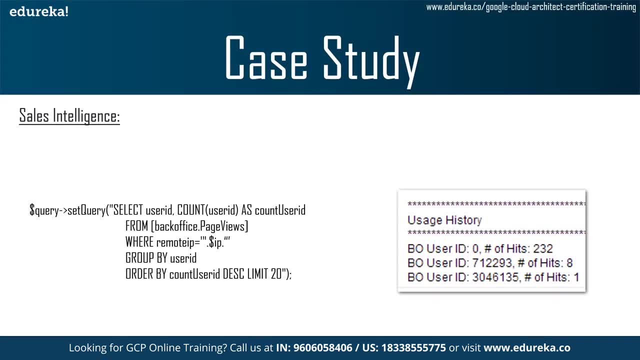 the analytics heavy lifting with a bigquery, then store the result in something like a cheap lamp stacks of mass consumption, and then the second advantage that the safari got through bigquery is sales intelligence, which is another use case. bigquery was great for covering safari's web. 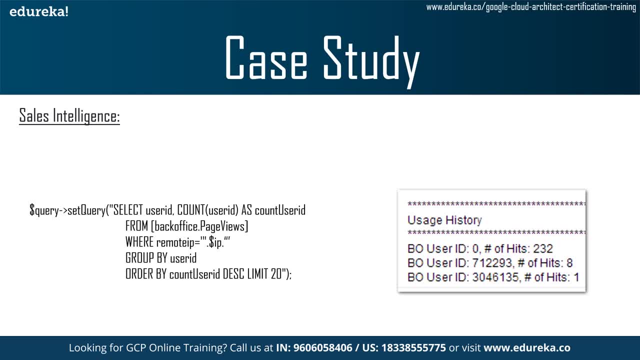 blocks for leads which came into their sales intelligence. and then the second advantage that the safari got through bigquery was that it was able to track the leads of the sales department. this allowed them to relate a leads to another accounts in the system or cause the level of 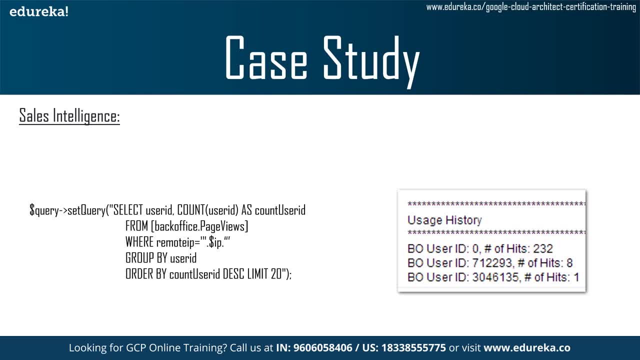 interest someone may have in safari by the number of previous book they had read in the past months. on their sites. elite is created in crm system and the bigquery asynchronously searches through its logs like this: so you can see this in query. like you can see the query written. so the result is: 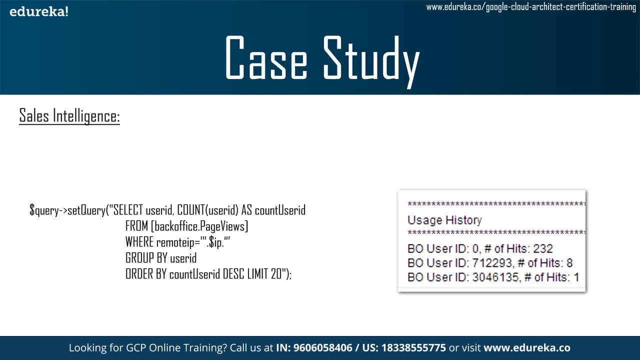 written quickly and reattached to the lead recorded, allowing safari sales department to gain intelligence without having to wait around the information. this give them a nice summary of the users: the ip address of the leads. that has been done. while ip address are not perfectly identifiers, they are much better. 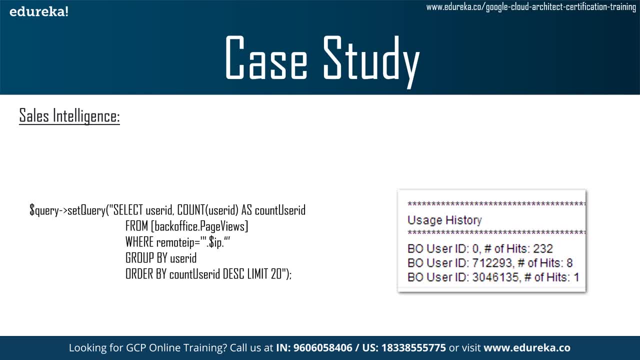 than nothing. you can see someone from this lead id. you can see its usage history. then see how it is given. so you can see someone from the lead ip address. has an anomalously view user id. 0 to 322 pages of a book and some other users who have accounts with safari already are active on that id. 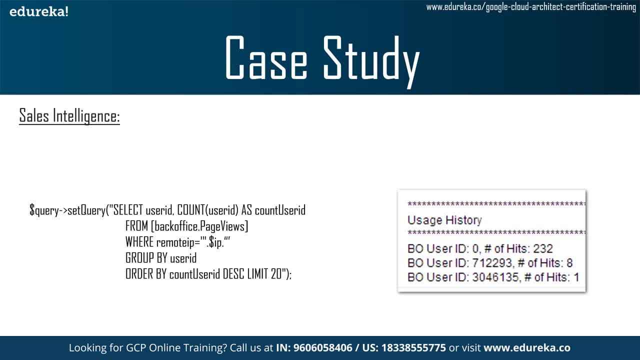 and then use the bigquery command line interface. this use case was better suited for server to server, or we say, or with an oort, which is like the authorization tool google even uses. so with the google apis client library for php. now this enables them to create web services. 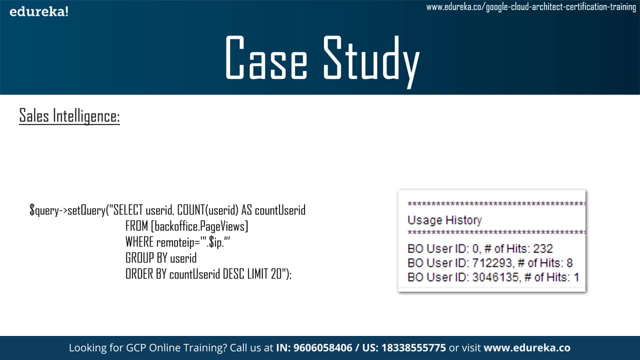 which match up data from different sources and return the result to the crm. one of the sources is the bigquery. one amazing testament to the speed of bigquery is the speed of bigquery that it didn't have to implement the web service asynchronously. now it returns the result from: 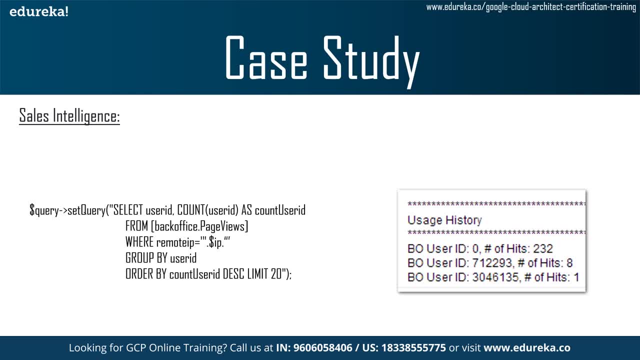 bigquery within the timeout period of the web service. that the crm requests at the use case of safari, which they took advantage of through using bigquery, is pure ad hoc querying which aren't driven by dashboard but rather specific business questions. when safari releases the android app, it was easy to run a query on our usage data and so on. safari usage data to see. 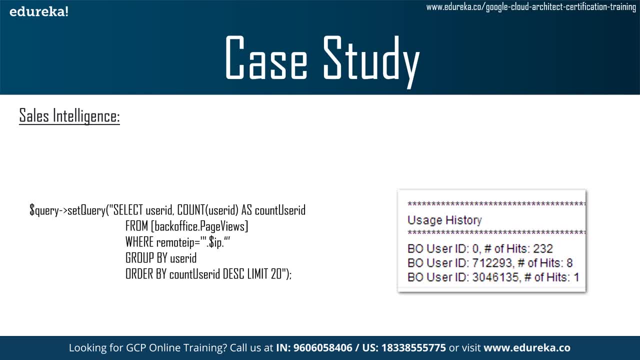 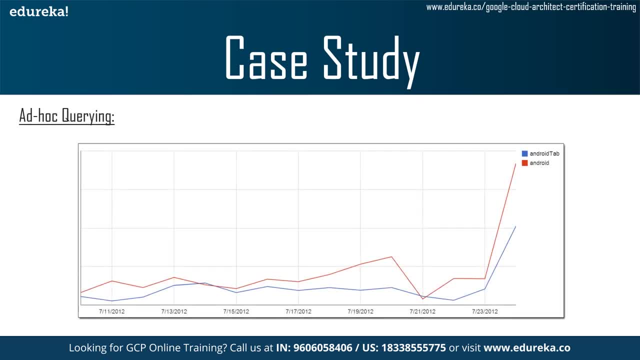 this show when this release their android apps. this is the graph and here's an example of looking at the top users by number searches during a particular hour of the day. there really is no limits to the kinds of insight you can gain from the investigation of data. from an ad hoc perspective, this is an actualization of the investigation regime for unsolved dépist. Anfang nach اقل. linux gut problems are ground, lost and caused byгов, browser cores and virtual app purchases. don't introduce our experts for the use case. 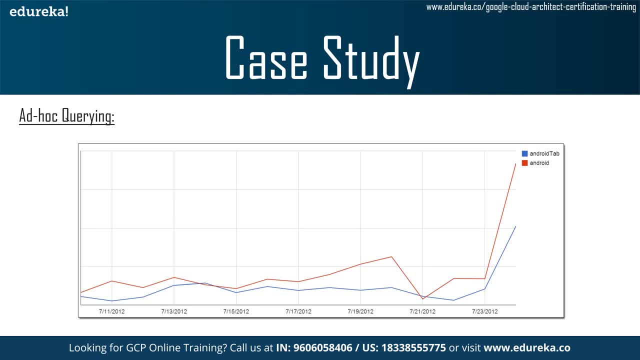 great tool is the high speed forskling tool, which can해x XML to arrive at the most simpleоль hou markupsbiqa. incorporation of tools, week to weekai storage apps, a huge sense of power, being able to answer any question about your millions of rows and. 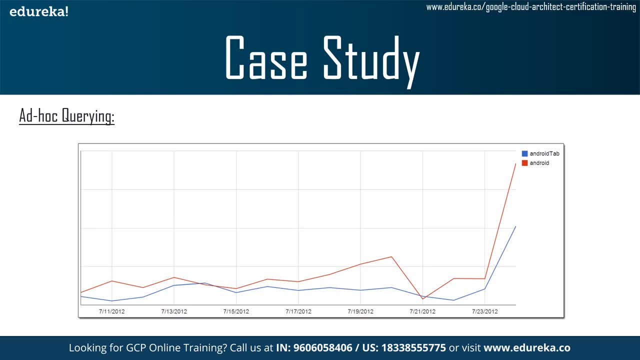 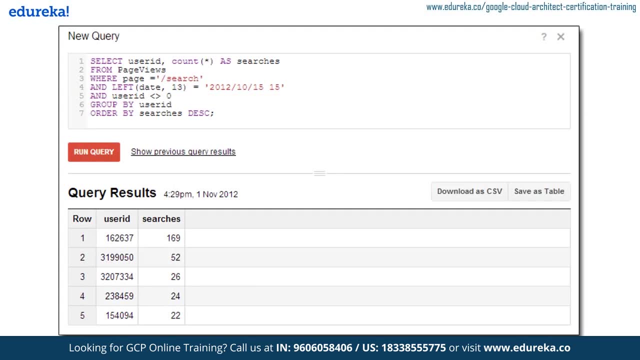 data in seconds. For example, you can find out if that strange traffic on your site is a foreign spam bot or a malicious user. as recommended by Google, They divided the data up into yours. You can see this in the table. Normally, this will be a bit of an inconvenience.